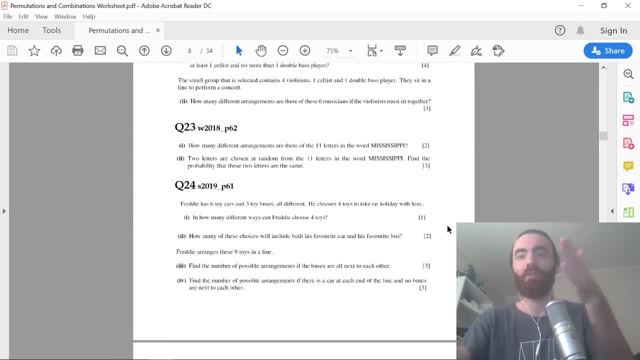 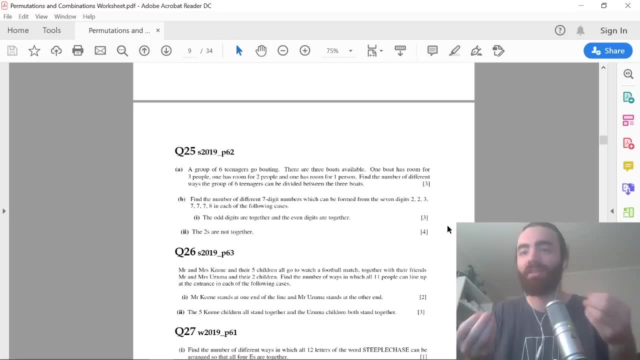 all from five years ago. There's 30 different questions, 30 different questions. So you go through the questions and you start to get a feel for how they like to ask this question. And let's say, if you don't know how to do it, well then you look at the answer. 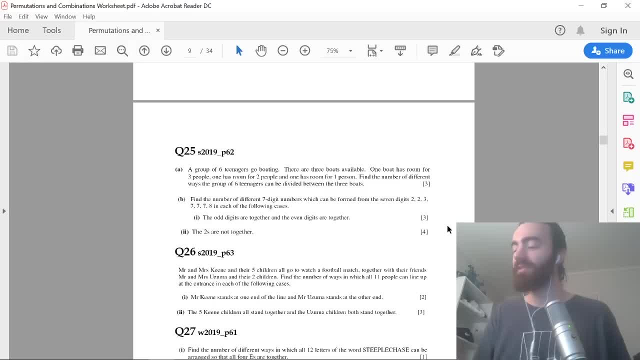 and you see that you've got it wrong and you're like, oh shit, Well then you spend the time to try and figure out the answer, Try and understand the answer, And once you understand the answer, then you can retry the question and get it right. And let's say, you just can't. 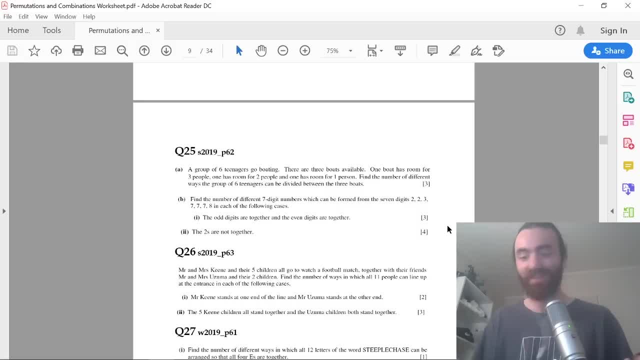 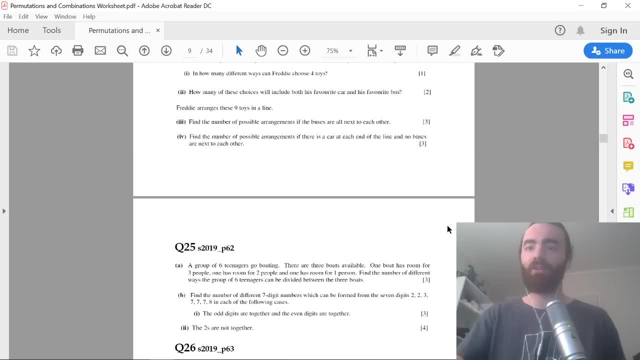 understand the answer. Well, use this resource, Use the comment section. Go ahead and write a comment, Go down there and ask: hey, I was doing question 25 on the worksheet and I couldn't do B, I just couldn't do it. And can you help me and help each other, And I'll be there and I can. 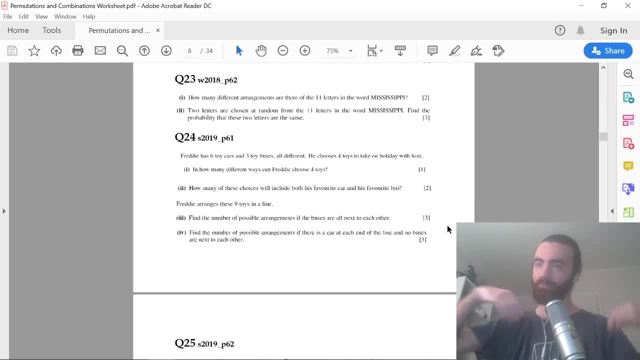 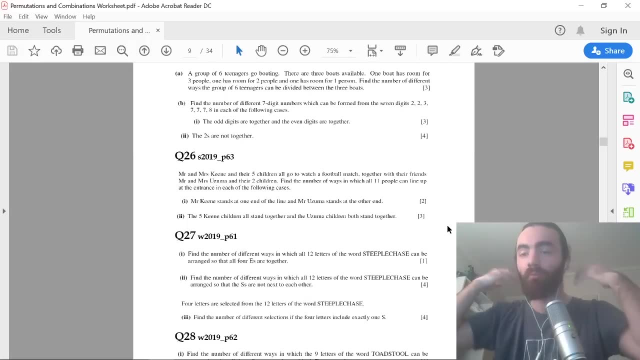 help as well, because it seems like you guys do struggle with this question. So you've got all of them there and go through them and you'll get a good idea. Your brain is so good at recognizing patterns When you go through this. your brain is so good at 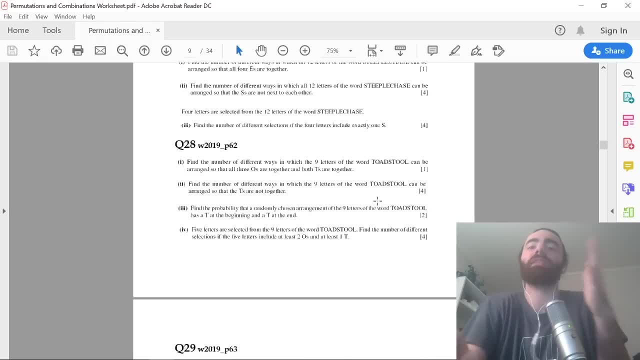 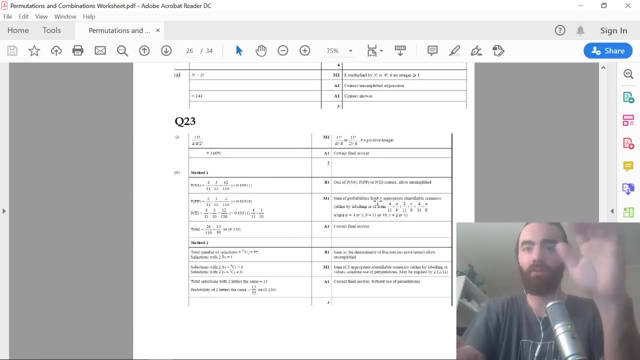 recognizing patterns. You'll see, You just get a feel for it. I can't really explain it Anyway. so you've got them there, So start going through them and getting an idea. And you've got all the extracted answers. And for the 2019 questions, I wrote my own answers for you, So you've got those there. 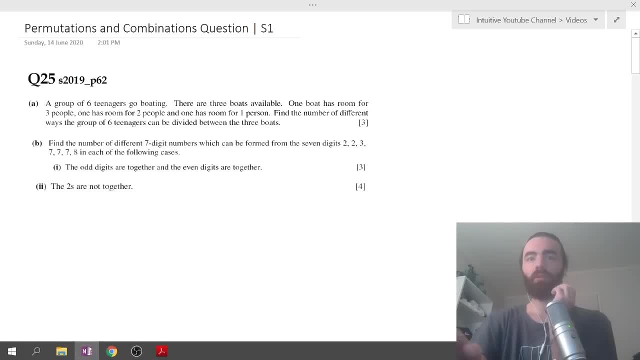 But really, in this video, what I'm just going to go through is, you know, a couple of questions from 2019.. Yeah, So we're going to go through those, I mean, and I guess, maybe before I do go through them, 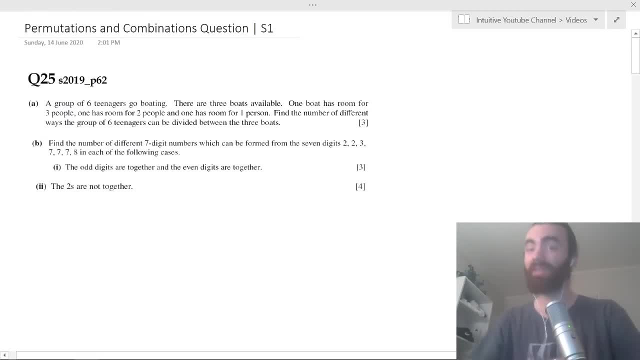 I'll just quickly show you, like, what the difference is between a permutation and combination. So really brief. So if you have three objects, ABC, well there is six permutations of this, which means there's six different ways for you to arrange this, or three factorial And 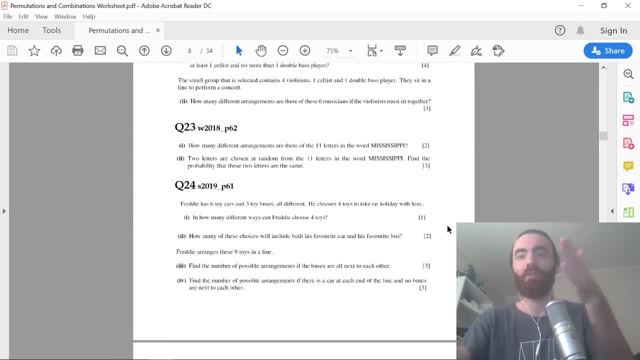 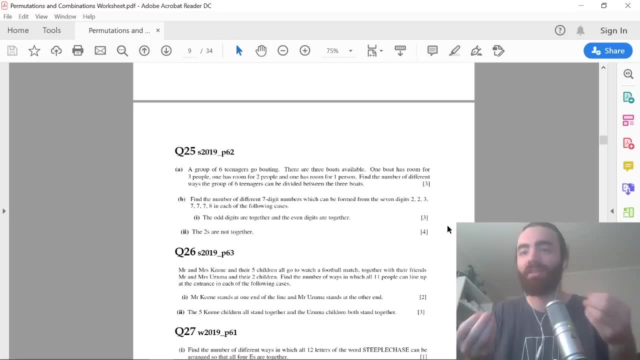 all from five years ago. There's 30 different questions, 30 different questions. So you go through the questions and you start to get a feel for how they like to ask this question. And let's say, if you don't know how to do it, well then you look at the answer. 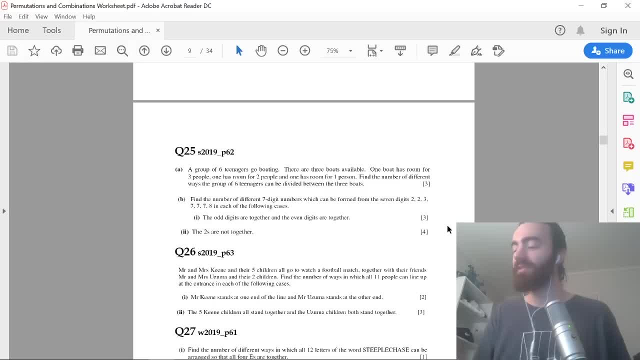 and you see that you've got it wrong and you're like, oh shit, Well then you spend the time to try and figure out the answer, Try and understand the answer, And once you understand the answer, then you can retry the question and get it right. And let's say, you just can't. 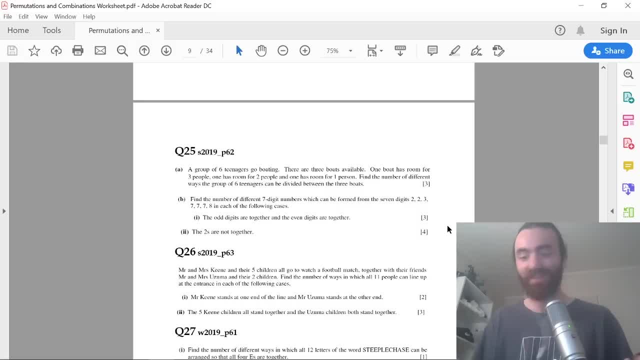 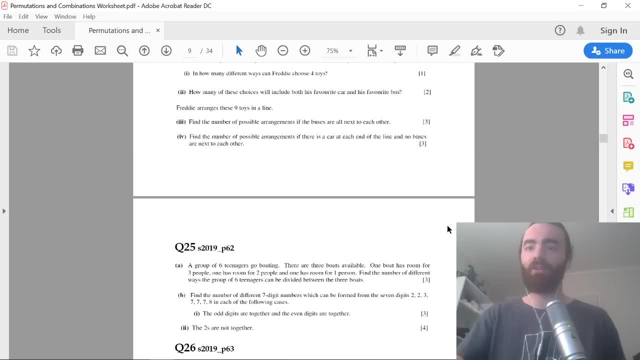 understand the answer. Well, use this resource, Use the comment section. Go ahead and write a comment, Go down there and ask: hey, I was doing question 25 on the worksheet and I couldn't do B, I just couldn't do it. And can you help me and help each other, And I'll be there and I can. 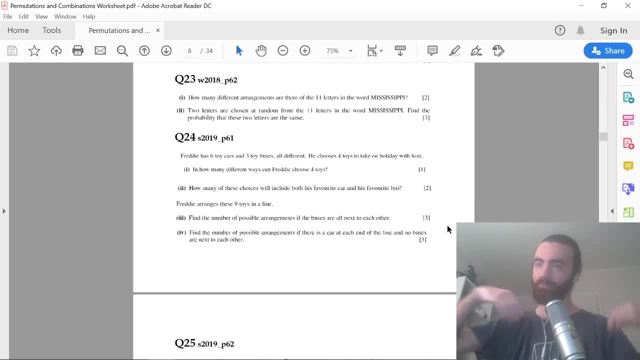 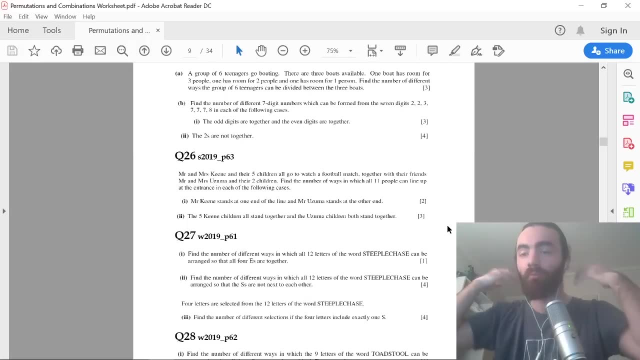 help as well, because it seems like you guys do struggle with this question. So you've got all of them there and go through them and you'll get a good idea. Your brain is so good at recognizing patterns When you go through this. your brain is so good at 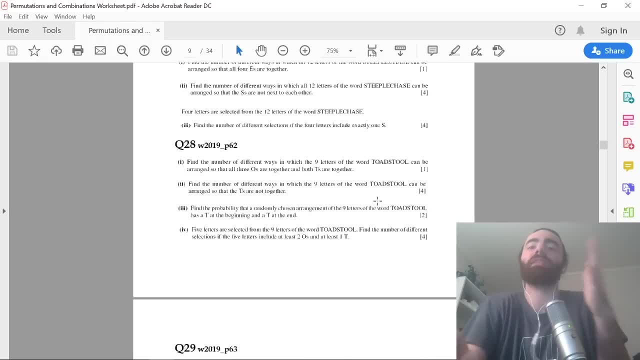 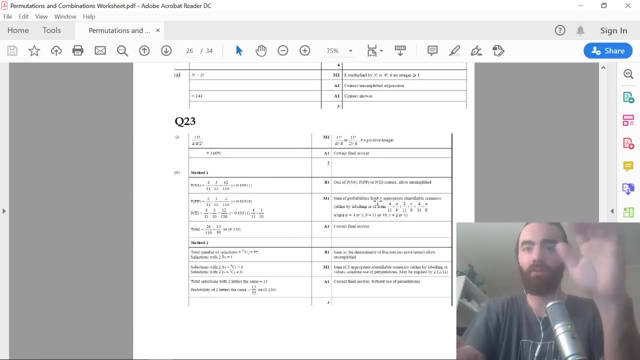 recognizing patterns. You'll see, You just get a feel for it. I can't really explain it Anyway. so you've got them there, So start going through them and getting an idea. And you've got all the extracted answers. And for the 2019 questions, I wrote my own answers for you, So you've got those there. 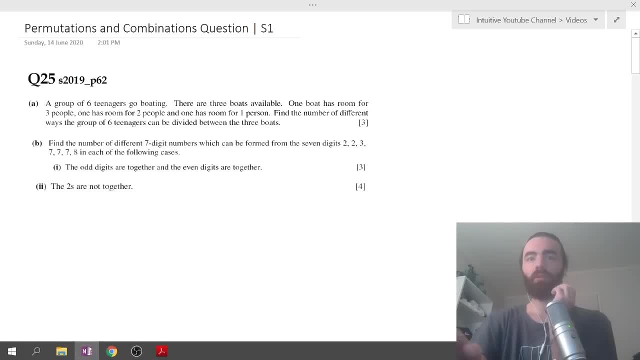 But really, in this video, what I'm just going to go through is, you know, a couple of questions from 2019.. Yeah, So we're going to go through those, I mean, and I guess, maybe before I do go through them, 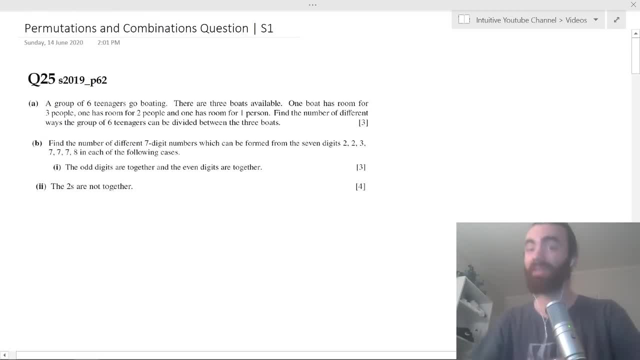 I'll just quickly show you, like, what the difference is between a permutation and a combination. So really brief. So if you have three objects, ABC, well there is six permutations of this, which means the six different ways for you to arrange this, or three factorial. 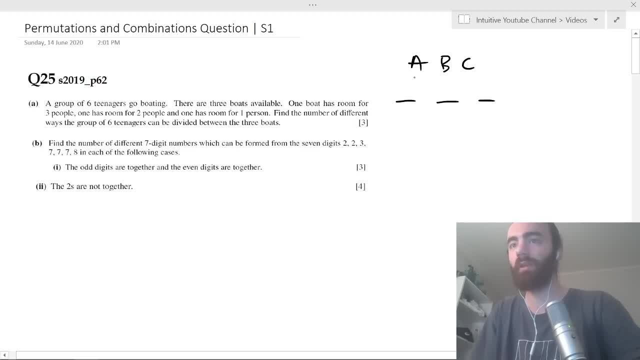 And the reason that that is is because, let's say, if you had three slots here, well, there's three different ways for you to select the first slot. You could pick an ABC and then, once you've picked one, there's then two letters. 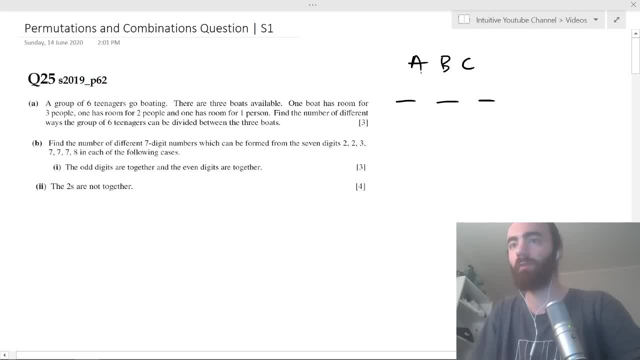 the reason that that is is because, let's say, if you had three slots here, well, there's three different ways for you to select the first slot. You could pick an ABC and then, once you've picked one, there's then two letters. 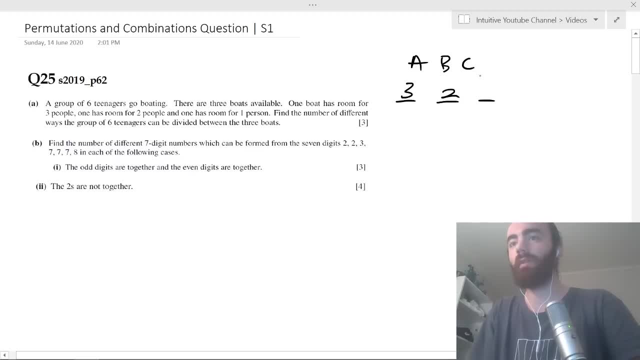 There's two different ways you can select the second spot, And then there's only one way you can select the third spot, And then you times it together. And the reason that you times this together is because, look, when you select the first one, there's then for. 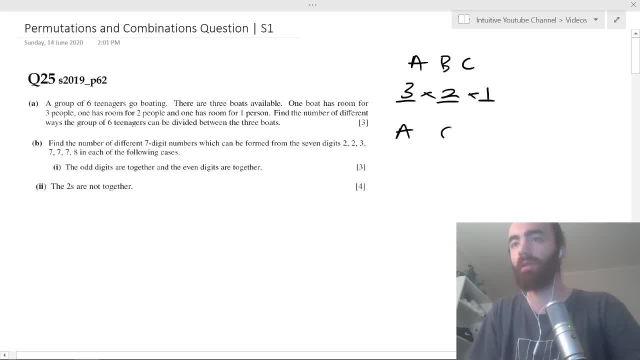 that one selection, there's then two different possibilities. And if you were to select B, there's then two different possibilities for the second one. That's why you multiply it. Okay, Cause you know, multiply whatever. that's why you multiply, And I hope that makes sense. 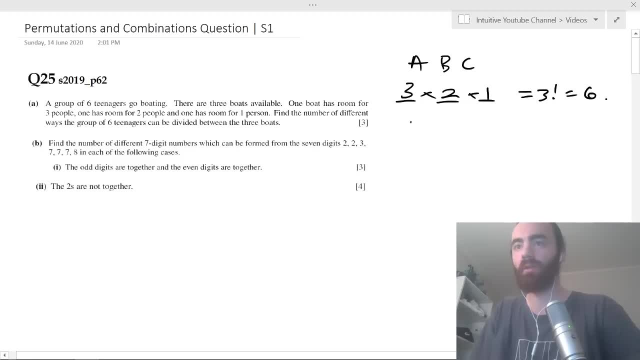 So that is equal to three, factorial, which equals six. So there's six different permutations, you know it's could be ABC, could be a ACB, could be BCA, And you know you get the idea. but there's only one combination, because in combination 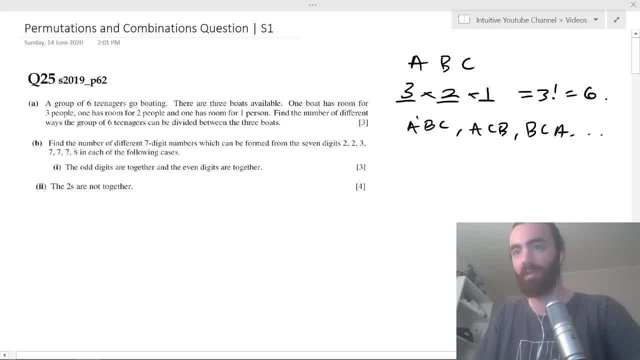 order doesn't matter. So for the, for the permutations, the order matters. right, This is different from this. We count them differently as a different arrangement, Whereas for combinations we do, the order doesn't matter. So these for a combination are all equal to this. over the. 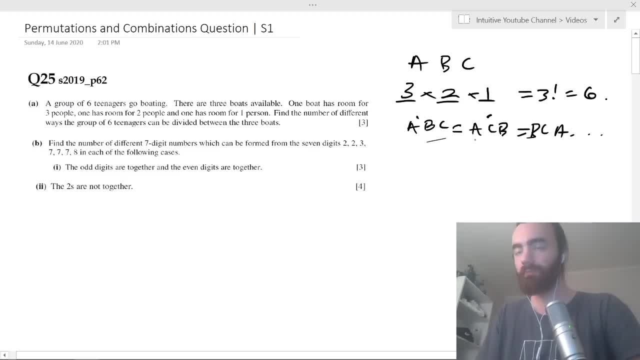 same. We say that the same set of objects, you know. so there's only one combination for this, but there's six permutations, Okay, So I hope that makes sense. Just thought I'd touch that briefly, but there's heaps of videos out there. 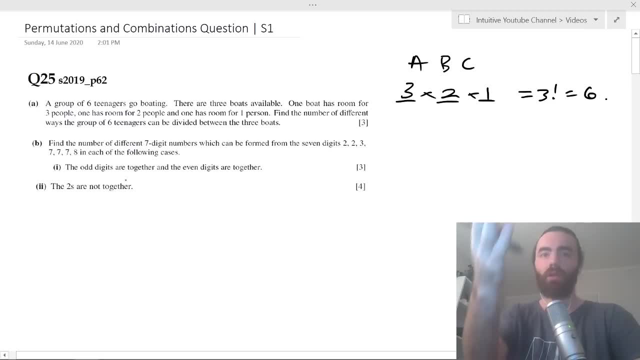 for you to go and understand this. Okay So, but what we're going to do, we're going to do some questions. you know, we've got this one and we've got another one here and they're pretty big questions from 2019.. You know, this is what this is: 11 marks. It's a pretty 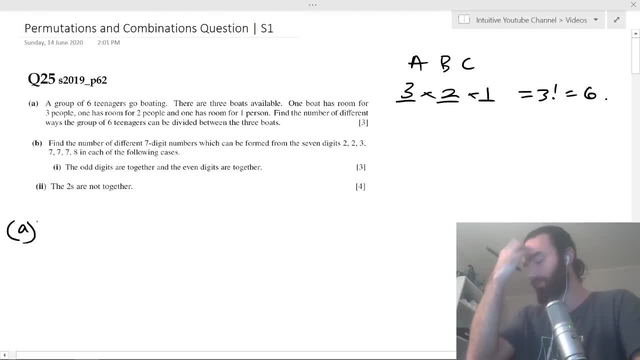 big question. Okay, And I'm going to explain them. I'm going to go into my thought process, like I say all the times, many ways to do this do these types of questions the way that I see fit to do it. Okay, So we've got a group of six teenagers and they're going. 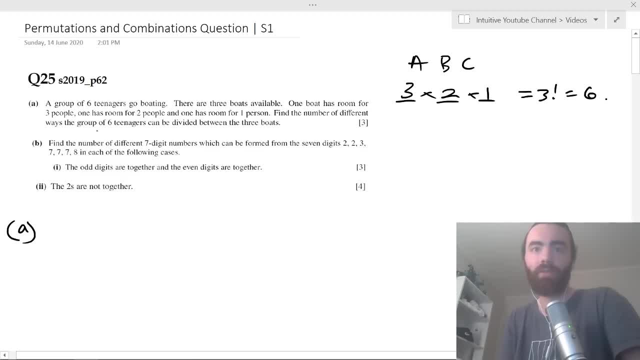 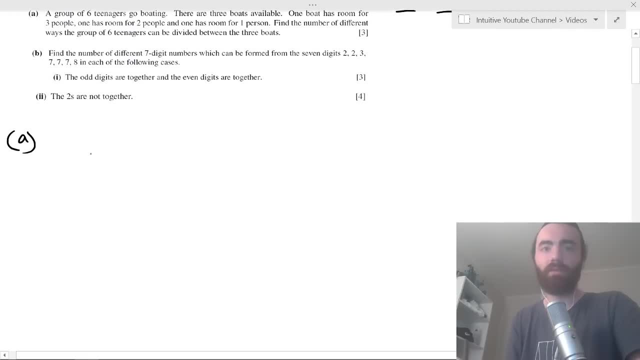 boating and there are three boats. One boat has room for three, one has room for two and one has room for one. Find the number of different ways The group of 16 years can be divided into three boats. Okay, So we have six teams, six individual teams. you know, not every. 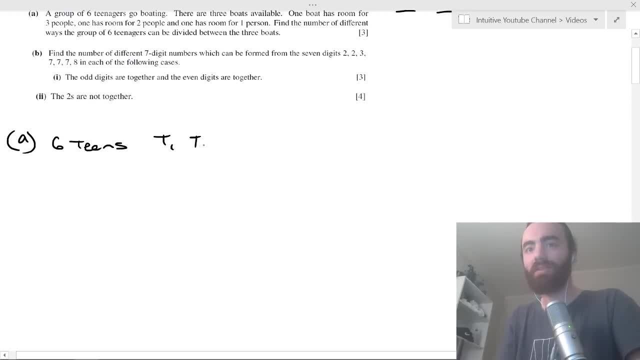 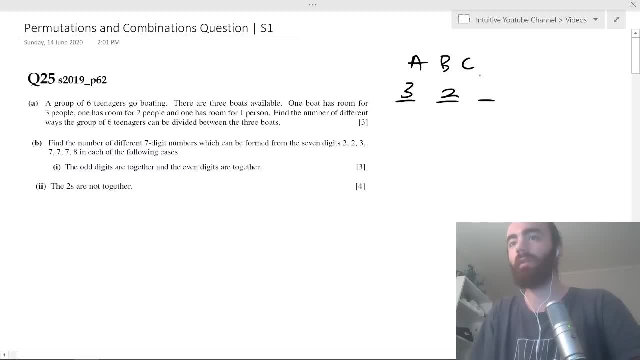 There's two different ways you can select the second spot, And then there's only one way you can select the third spot, and then you times it together. And the reason that you times this together is because, look, and when you select the first one, there's then 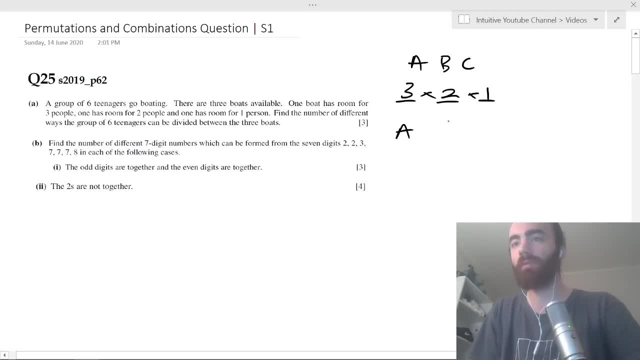 for that one selection, there's then two different possibilities. And if you were to select B, there's then two different possibilities for the second one. That's why you multiply it. Okay, Cause you know, multiply whatever. that's what you multiply, And I hope that makes sense. 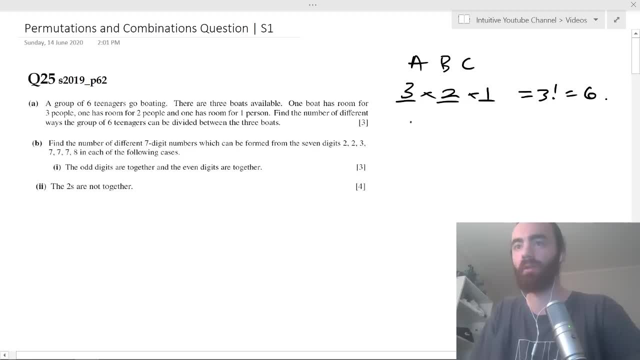 So that is equal to three, factorial, which equals six. So there's six different permutations. you know this could be ABC, could be a ACB, could be BCA, And you know, you get the idea. but there's only one combination, because in combination 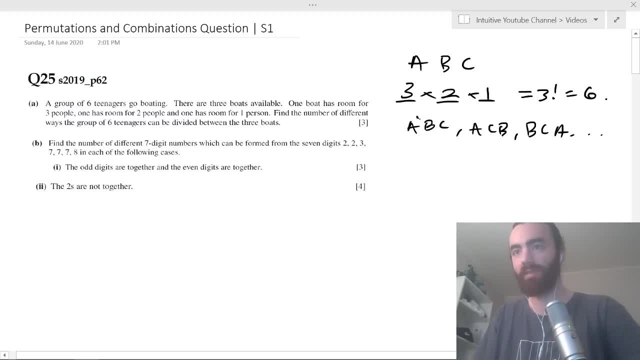 order doesn't matter. So for the, for the permutations, the order matters. right, This is different from this. We count them differently as a different arrangement, Whereas for combinations we do, the order doesn't matter. So these for a combination are all equal to this. over the. 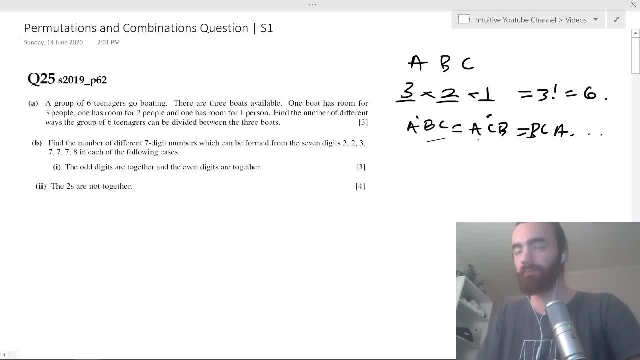 same. We say that the same set of objects, you know. so there's only one combination for this, but there's six permutations, Okay, So I hope that makes sense. Just thought I'd touch that briefly, but there's heaps of videos out there. 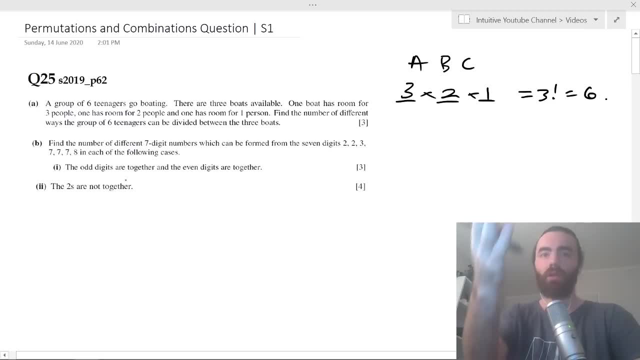 for you to go and understand this. Okay So, but what we're going to do, we're going to do some questions. you know, we've got this one and we've got another one here and they're pretty big questions from 2019.. You know, this is what this is: 11 marks. It's a pretty 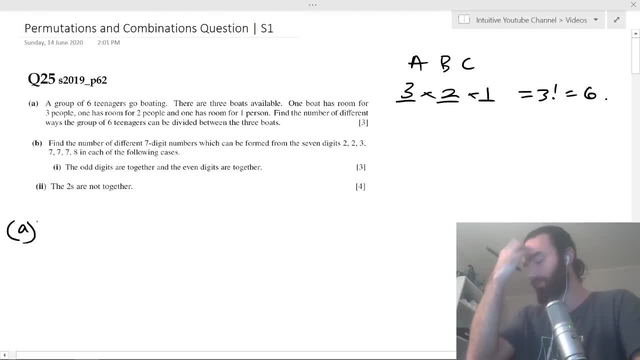 big question. Okay, And I'm going to explain them. I'm going to go into my thought process and, Like I say all the times, many ways to do this, do these types of questions the way that I see fit to do it. Okay, So we've got a group of six teenagers and they're going 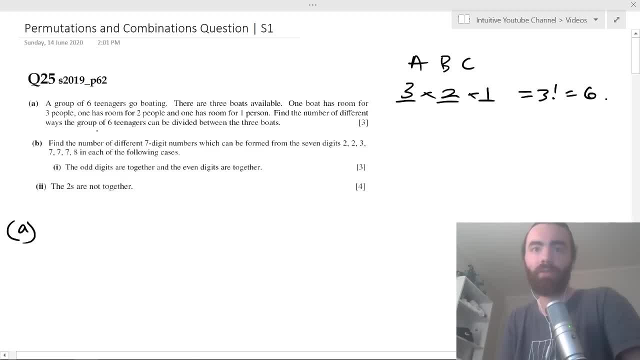 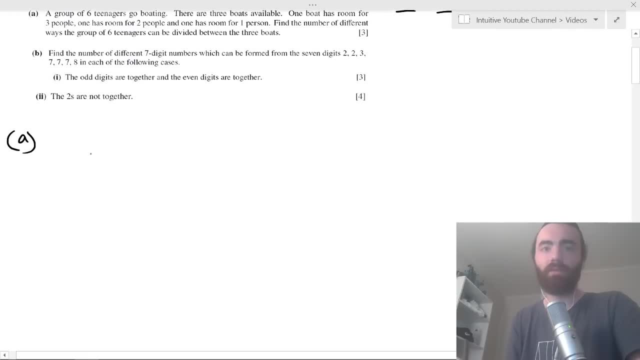 boating and there are three boats. One boat has room for three, one has room for two and one has room for one. Find the number of different ways The group of 16 years can be divided into three boats. Okay, So we have six teams, six individual teams. you know, not every. 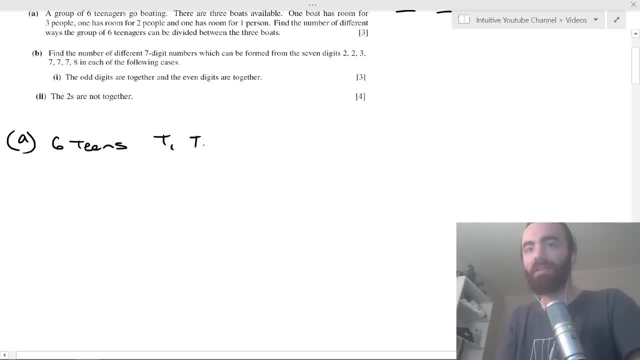 teenager is the same. Uh, let's call them T one, T two, T three, T four, T five And T six. you know six different teams And we've got this first boat which has three slots, or three, um uh, places for the teenagers to sit. So this could be part one, And then 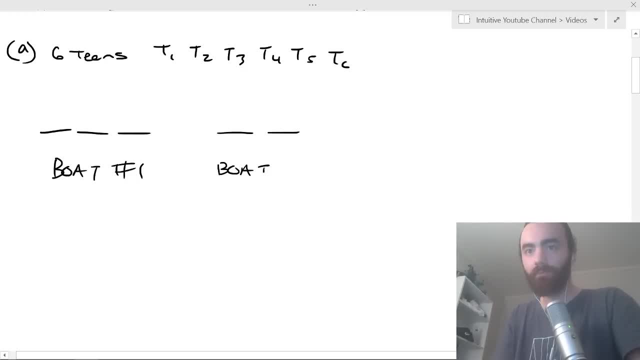 the second one has two places open, So that's boat two. And then the final one has only one boat, boat three. Okay, So how many different ways can this happen? Well, for the first boat, let's say, if we start with the first boat, well, how many if we have six teenagers? 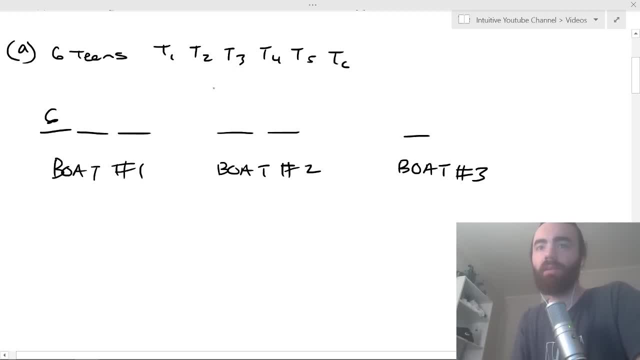 how many different ways can they sit in this boat? Well, you have six selections You can make. six different people can sit in the first one, and then five different people- cause you've taken one away- can sit in the second one, And then- um sorry, four different people. 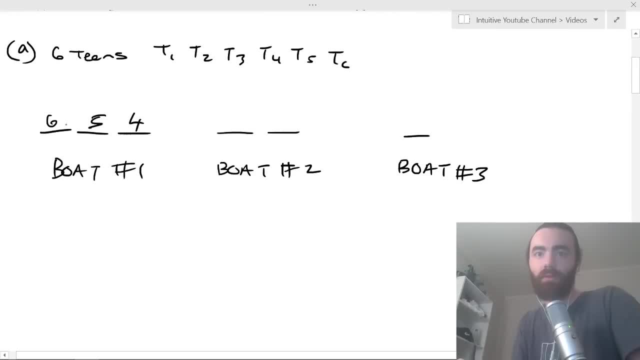 can sit in the third one And, like before when I said that these are obviously multiplied together, you know, but- and really this is the important thing about this question is you have to take into account when you're over counting and you are over counting it. 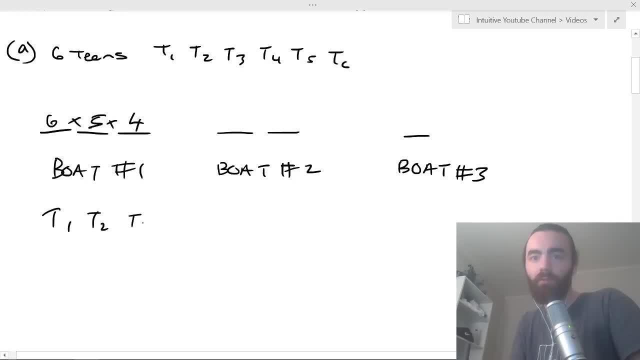 because you're saying T1,, T2, T3, right, If you pick that for these three things, you're counting that. And then you're also counting well. let's say, if I pick T2,, T1, T3, and you're saying well, 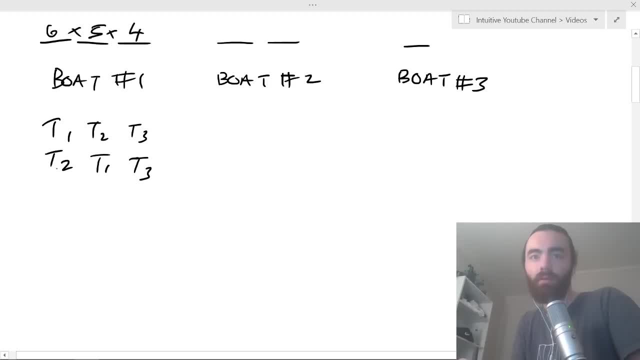 that's also a selection, But in fact that that's the same selection the same. there's two permutations, one combination. that's the same selection. right, There's the same set of teenagers sitting in boat one. You know, it doesn't matter where they sit, That's. 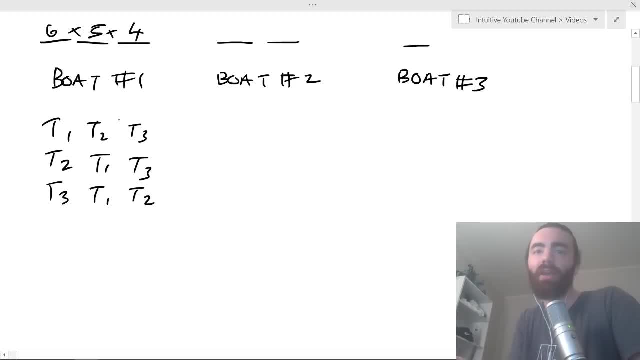 what I'm saying. Okay, So we have to divide, Okay, By three factorial, because this is the number of ways that we can arrange these three objects. So for the first boat we have six times five times four, divided by three factorial. Okay, 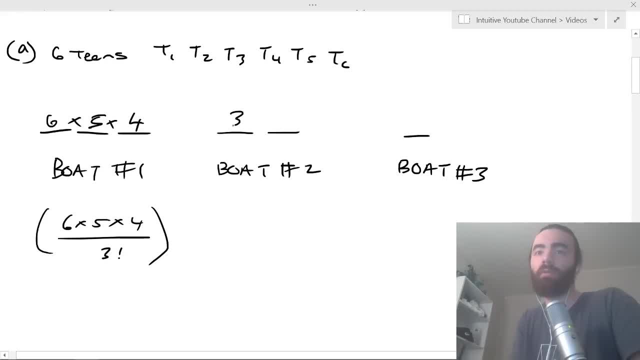 And then for boat two. well, now we've only got three teenagers left, So we have three selections for the first one and two for the second one, So three times two. but again we could pick T2,, T1, or, and that would be the same as T1, T2.. So we need to divide by. 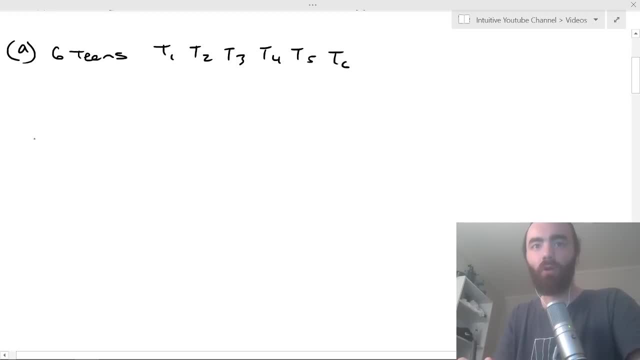 And T six, you know six different teams, And we've got this first boat which has three slots or three- um uh, places for the teenagers to sit. So this could be part one. And then the second one has two places open, So that's boat two. And then the final one has only 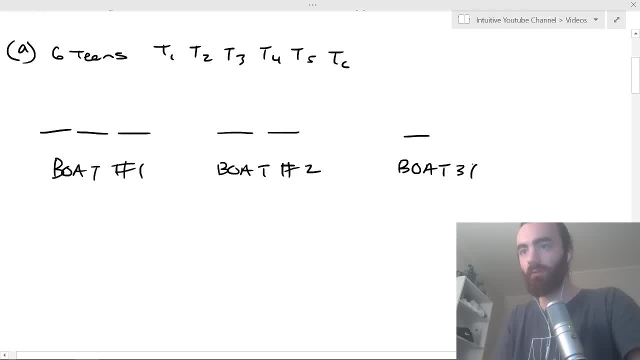 one boat, Oh, boat three, Okay. So how many different ways can this happen? Well, for the first boat, we start with the first boat. Well, how many? if we have a six teenagers, how many different ways can they sit in this boat? Well, you have six selections. You can make six different. 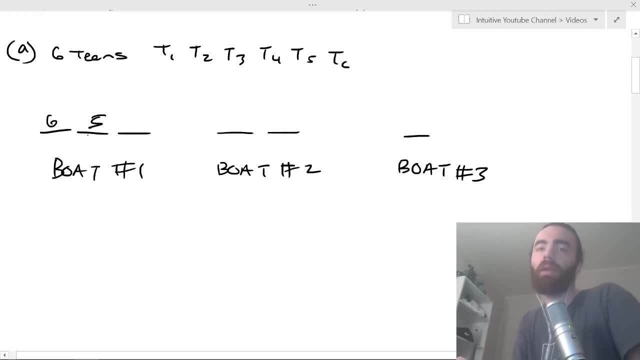 people can sit in the first one, and then five different people- cause you've taken one away- can sit in the second one, And then, um sorry, four different people can sit in the third one. And, like before, when I said that these are obviously multiplied together, you know. 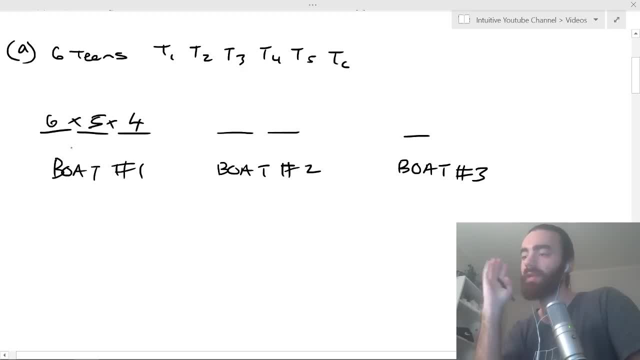 but- and really this is the important thing about this question- is you have to take into account when you're over counting. and you are over counting it because you're saying T1, T2,, T3, right, If you pick that for these three things, you're counting that, And then 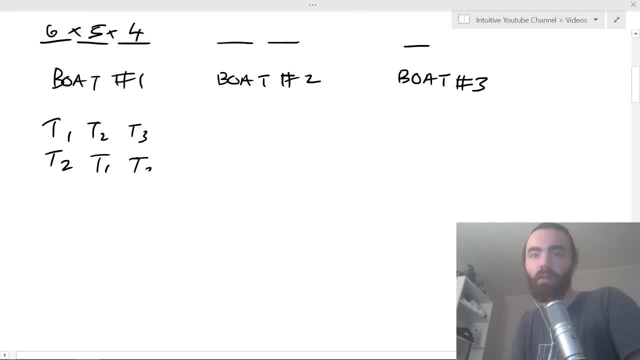 you're also counting. well, let's say, if I pick T2,, T1,, T3, and you're saying, well, that's also a selection, but in fact that that's the same um selection, the same as a car. 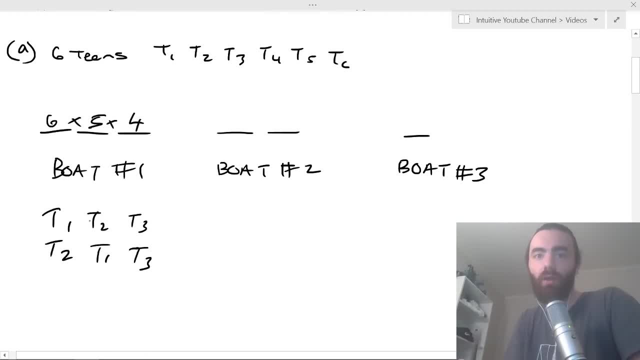 there's two permutations, one combination. that's the same selection. right, There's the same set of teenagers sitting in boat one. You know, it doesn't matter where they sit, That's what I'm saying. So we have to divide by three: factorial, because this is the number of ways that we can arrange. 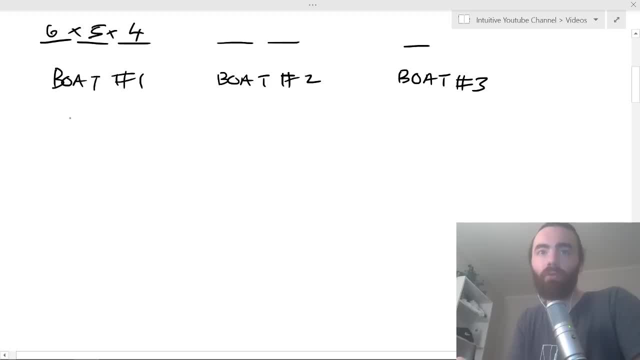 these three objects. So for the first boat we have six times five times four, divided by three, factorial Okay. And then for boat two, well, now we've only got three teenagers left. So we have three selections for the first one and two for the second one, So three. 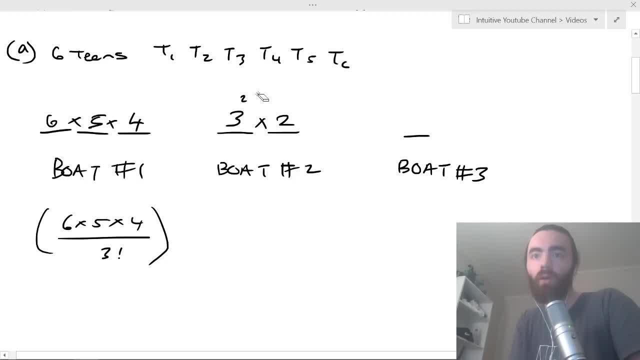 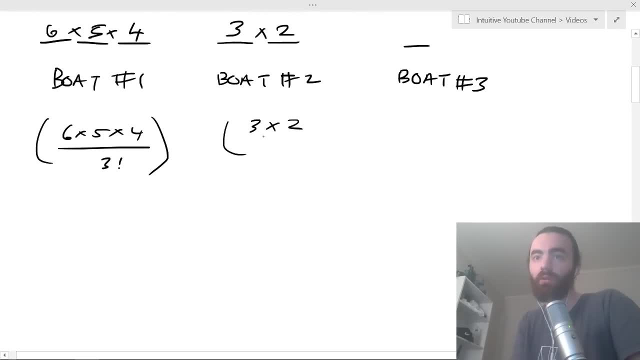 times two, but again we could pick T2,, T1, or, and that would be the same as T1, T2.. So we need to divide by the number of ways we can arrange. Uh, two objects, which is two factorial, And then for the last one, well you have. 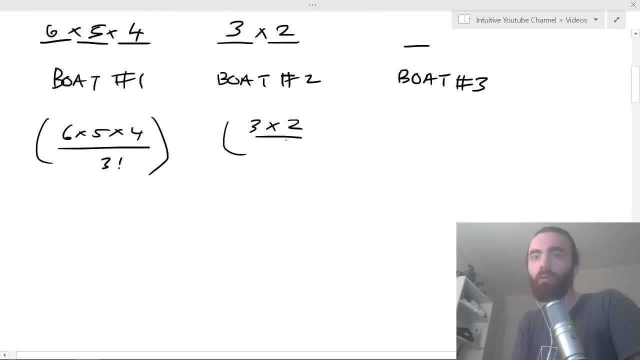 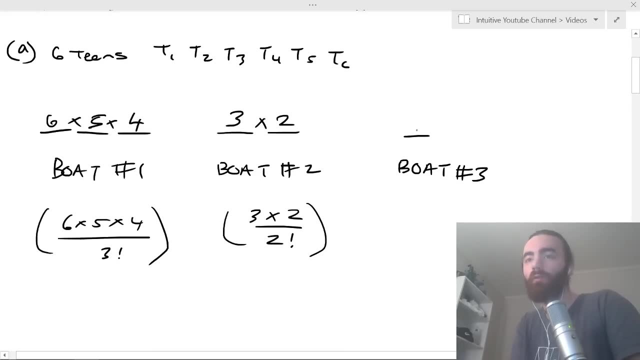 the number of ways we can arrange: uh, two objects, Okay, Which is two factorial. And then for the last one, well, you have uh only one teenager left, because we've already picked five, and you have one um slot left, right, So you. 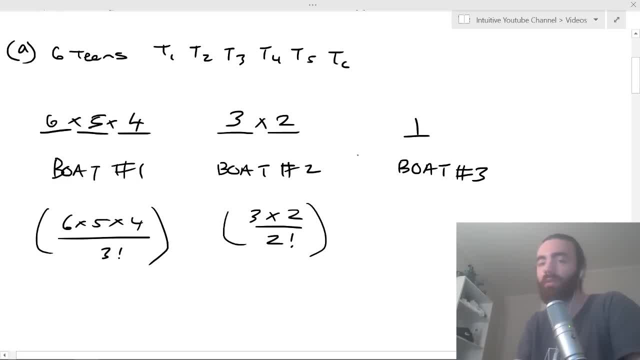 only have one. there's only one way to do that. I've got one dude and one slot. Well, there's only one arrangement of that, So there's only one here. And just to know, like, this is the same, um, you know this. this is the same as saying six, you know, from six objects. 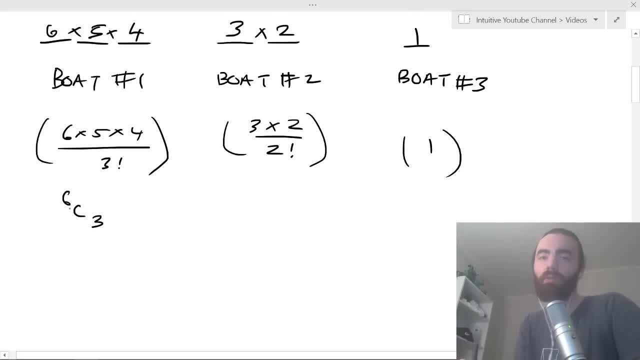 we are picking three. How many ways can we do that? How many combinations are there to do that? But I just like doing it this way. I don't know why it's just me: three C2.. This is the same as it'd be one C1, right, And we then? 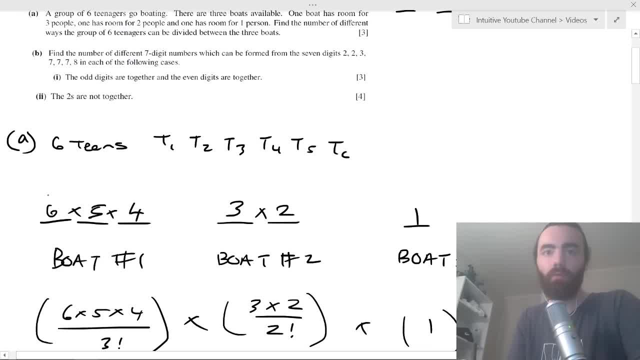 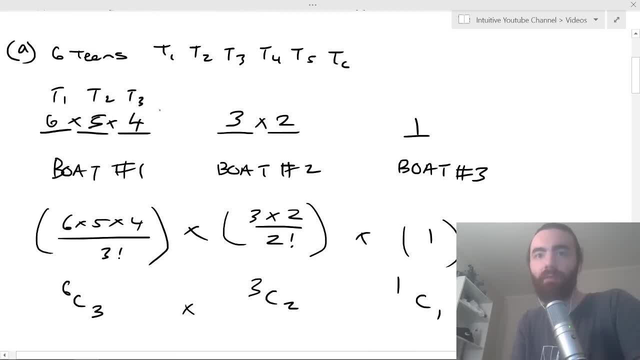 we multiply these together because you know, if you think about it, for one selection I make, let's say I make T1,, T2,, T3, and this might be a bit overkill- but the reason it's multiplied because then for that one selection there is then um this many. so this is what 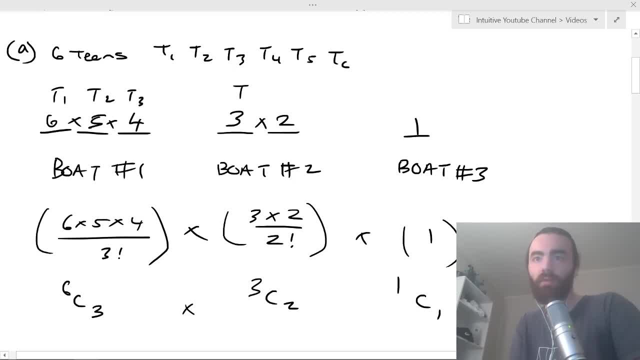 six divides And there's three different ways then. So there's this, three different ways to do it. Okay, So there's three different ways to select boat, two for this. one boat, one selection, So you could pick like T6, T4, you can put T6,, T5, you know this. those different ways. 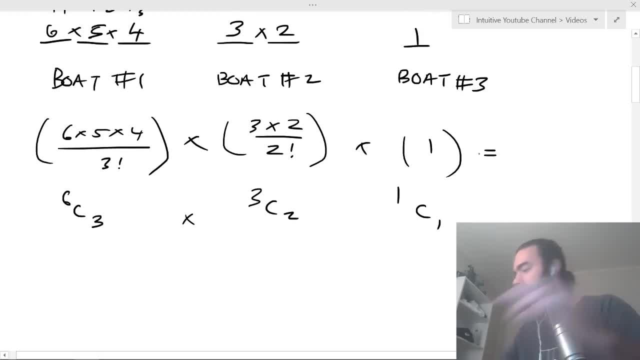 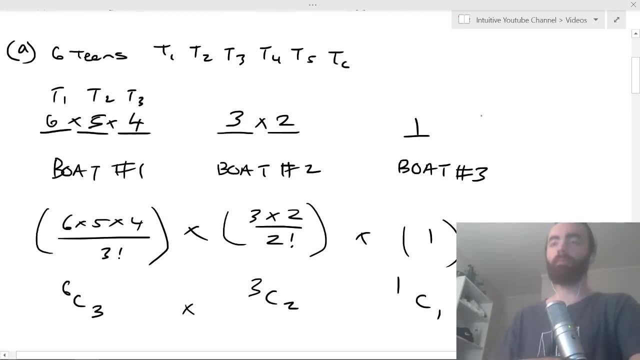 So that's why we multiply. So you multiply all those together and you'll get who times three, 60 wise you to get 60 ways. Okay, Okay, Okay, did it the other way around, like you started with boat one. i'll just do this real quick, like it. 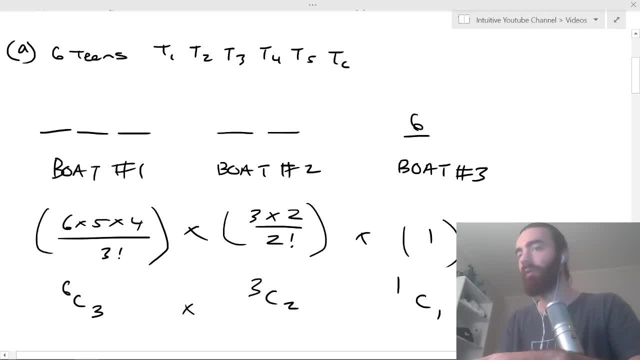 doesn't matter, like you started with one. okay, there's six ways here for you to pick boat one. i mean you start with boat three, sorry. well, there's six different ways here. times, six different ways here. times, how many here? well, there's five teenagers times four teenagers divided by two. 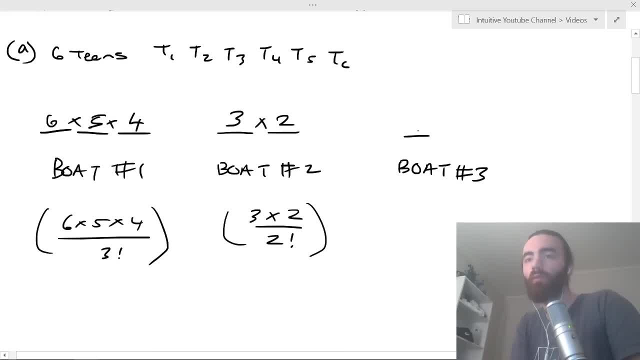 uh, only one teenager left, cause we've already picked five and you have one um slot left right, So you only have one. there's only one way to do that. I've got one dude and one slot. Well, there's only one arrangement of that. So there's only one here And just. 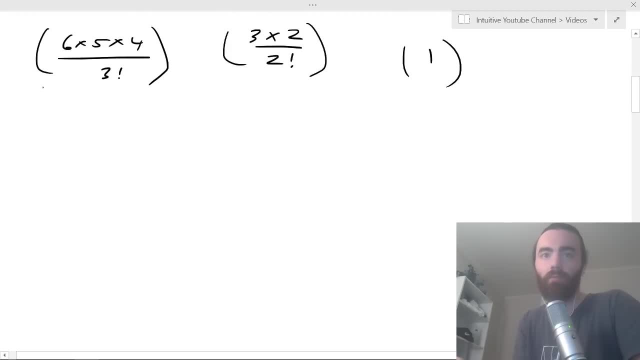 to know, like: this is the same. um, you know this. this is the same as saying six. you know, from six objects we are picking three. Okay, How many ways can we do that? How many combinations are there to do that? But I just like doing. 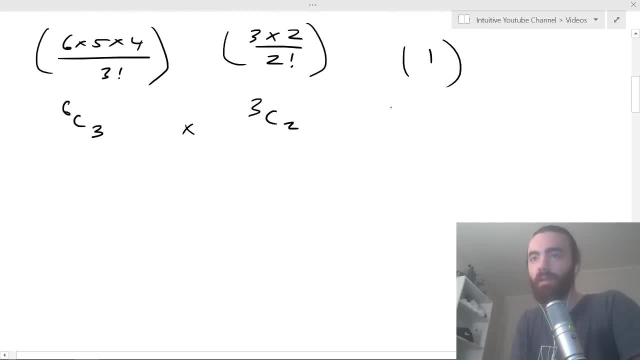 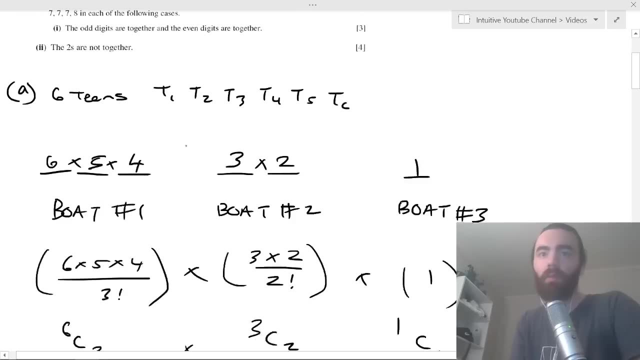 it this way, I don't know why it's just me- three C2.. This is the same as it'd be one C1, right, And we then we multiply these together because you know, if you think about it, for one selection I make, let's say I make T1,, T2, T3, and this might be a bit overkill. 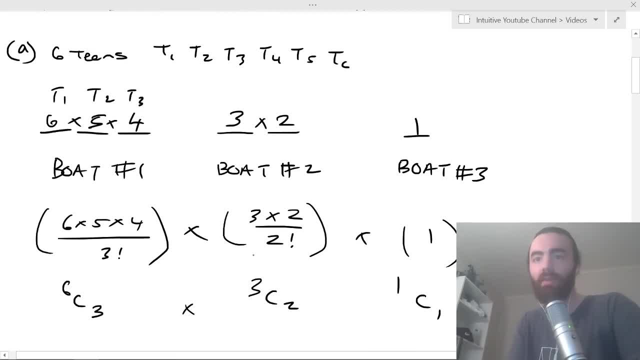 but the reason it's multiplied, because then for that one selection there is then um this many. So this is what six divides. So there's three different ways then. So there's this: there's three different ways to select boat two for this one boat, one selection. So you: 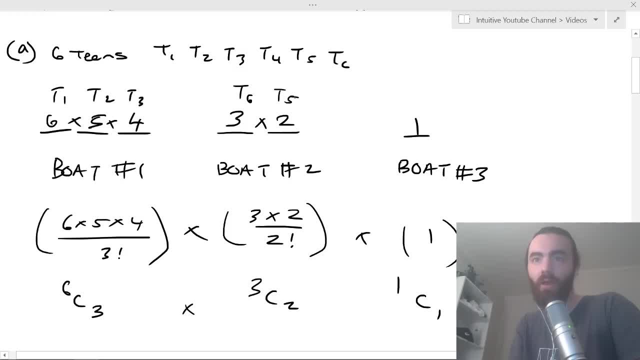 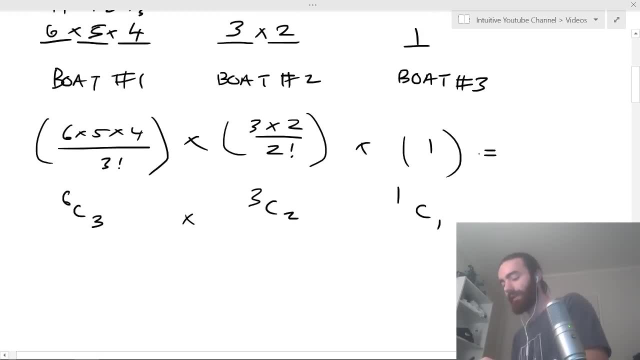 can pick like T6, T4, you can put T6, T5, you know this, those different ways. So that's why we multiply. So you multiply all those together and you'll get who times three, 60 ways, you to get 60 ways. Okay, And just to know if you get 60 ways. 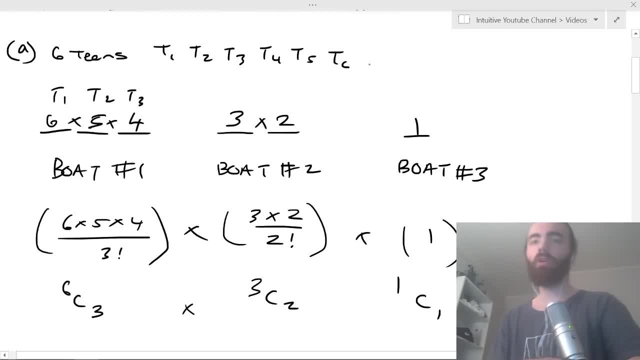 you're good to go, Okay. Okay, did it the other way around, like you started with boat one. i'll just do this real quick, like it doesn't matter. like you started with one. okay, there's six ways here for you to pick boat one. 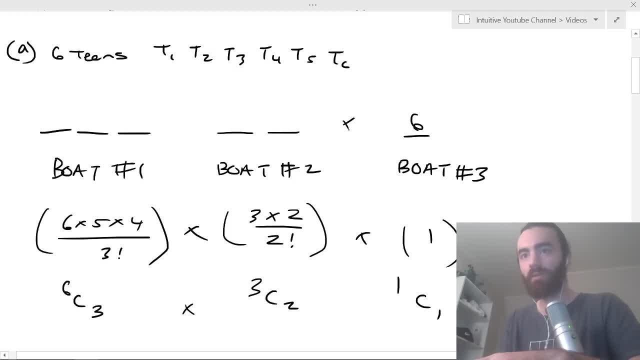 i mean, you start with boat three, sorry. well, there's six different ways here times. six different ways here times, how many here? well, there's five teenagers times four teenagers divided by two factorial times. here you have then a three times two times one, divided by three factorial well, 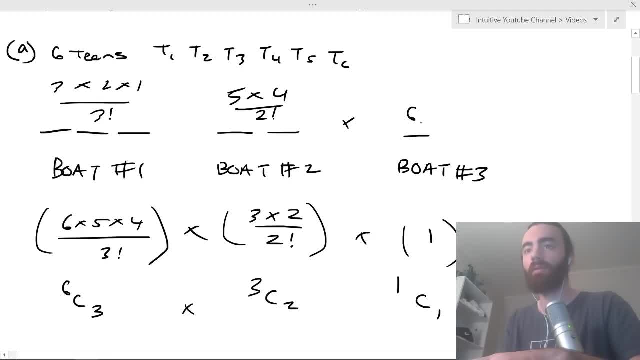 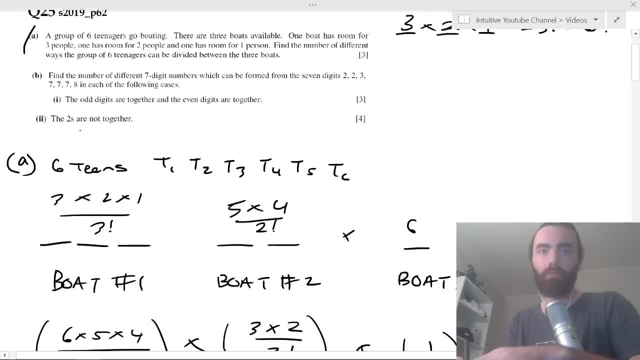 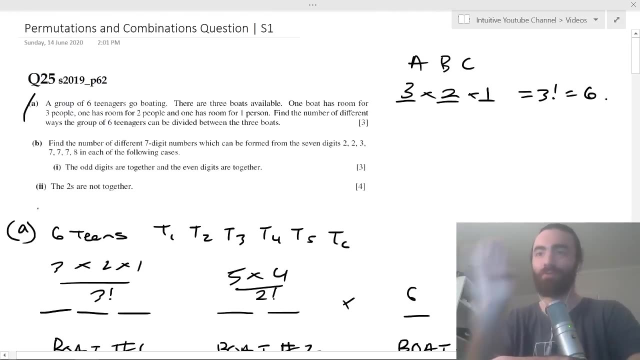 this is then one times ten times six, which is 60. you know, it doesn't matter which which makes sense, right, anyway, might have gone a bit overboard. cool when they ask things in this style all the time. man just go through. do start, just start doing questions on the worksheet. you got them. 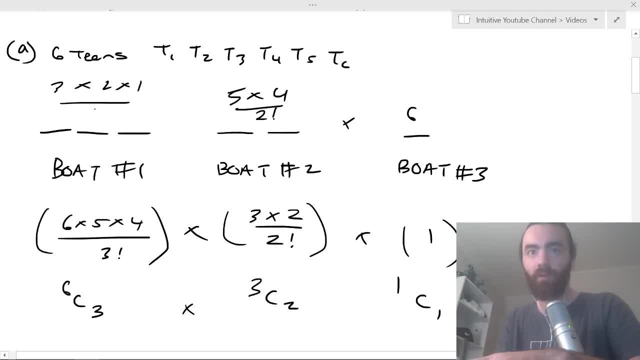 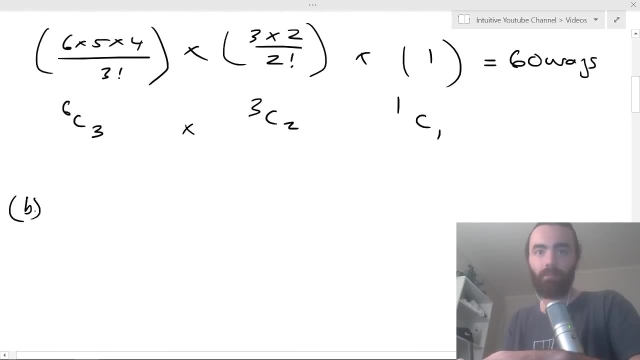 factorial times. here you have then a three times two times one, divided by three factorial. well, this is then one times ten times six, which is 60. you know, it doesn't matter which which makes sense, right, anyway, might have gone a bit overboard. cool, when they ask things in this style, all the 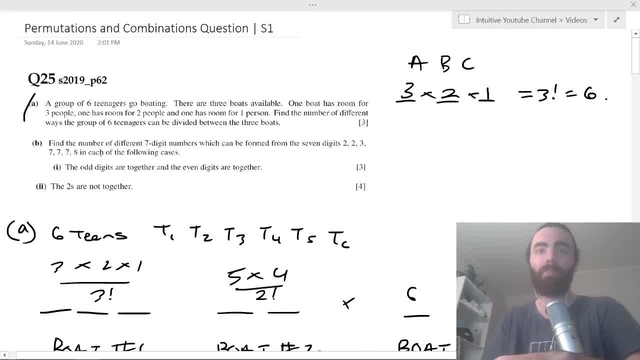 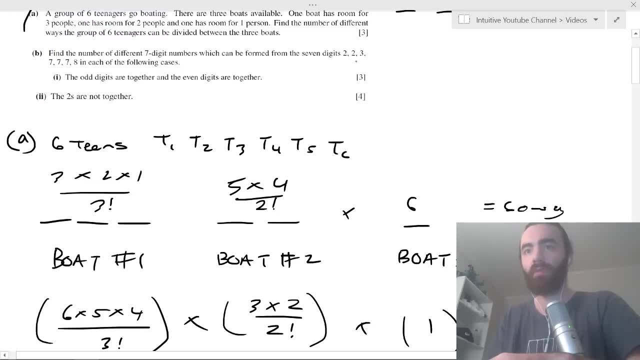 time, man, just go through, do start. just start doing questions on the worksheet. you got them all there and got all the answers. um, okay, so find the number of different seven digit numbers which can be formed from the seven digits two, two, three, seven, seven, seven, eight. you got them all there and got all the answers. um, okay, so find the number of different seven. 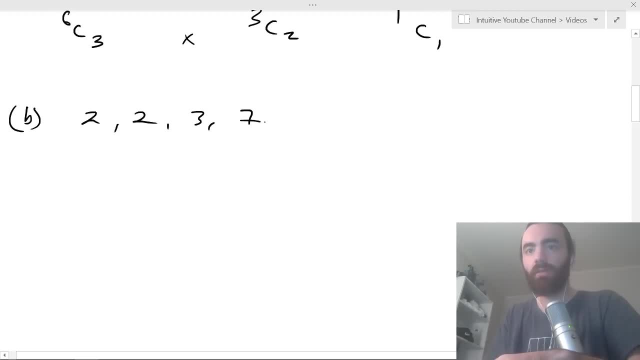 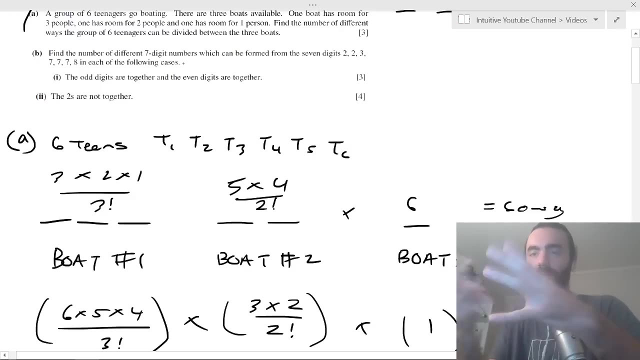 digit numbers which can be formed from the seven digits: two, two, three, seven, seven, seven, eight, okay, um, so it wants to know how many ways we can form different digits or arrange these numbers with certain limitations, and these limitations are for the first cases, for i, is that the odd. 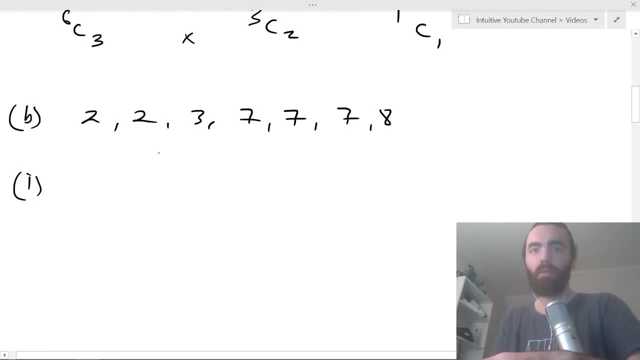 digits are together and the even digits are together. okay, so that means that all of the odd digits, the three, seven, seven, seven, that's together. this is how i like to think about it. we put them in like a one slot or one box. all right, this is like one slot. 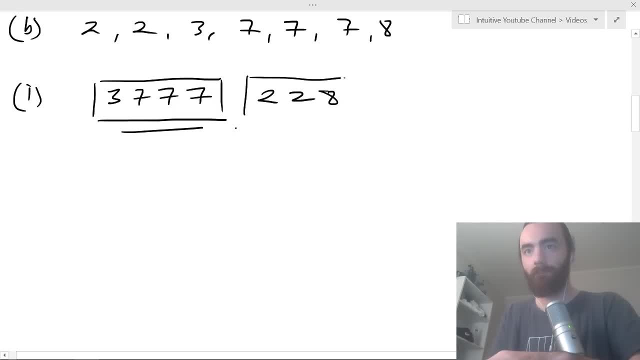 and then our second slot would be two, two, eight. okay, so then we can move these around two ways, right? so we can this three, three, i mean this three, seven, seven, seven could be in the first or the second, so there's two different ways for us for me to arrange that. so two times, well, how many ways? 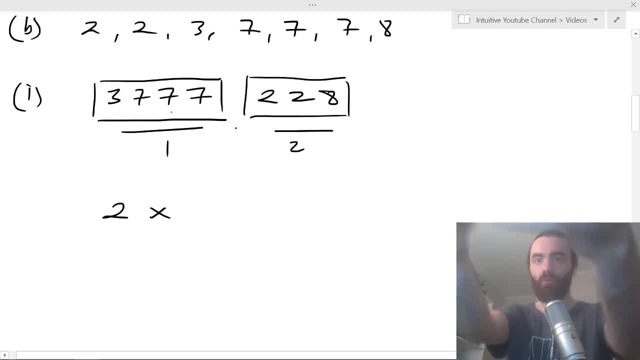 can i then arrange these um, the internal structure of these boxes, the internal digits, right? so let's say for this one, well, there's four objects, so it'd be four factorial ways. but again, we're over counting, because i'm, i'm, i'm counting the when i move these sevens. i'm saying that if we have three, three, seven as one, 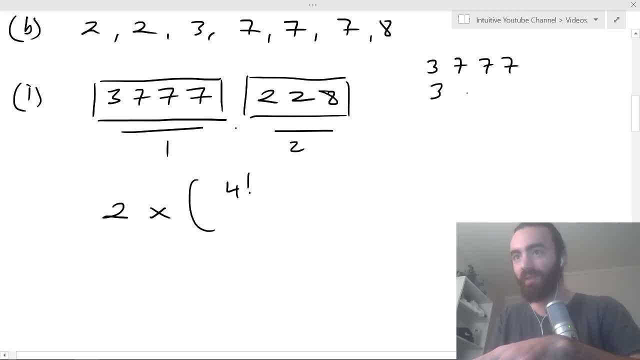 well, i'm also counting three and then i move these sevens around. so let's say i move this seven here, seven, seven, seven. but look, it's the same thing and i'm also counting when i move this seven with this seven, you know like. so i'm over counting, so i have to divide by the amount i'm over counting for each selection. 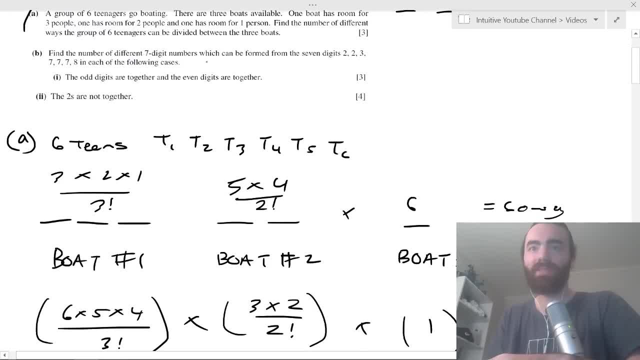 all there and got all the answers. um, okay, so find the number of different seven digit numbers which can be formed from the seven digits two, two, three, seven, seven, seven, eight. you got them all there and got all the answers. um, okay, so find the number of different seven. 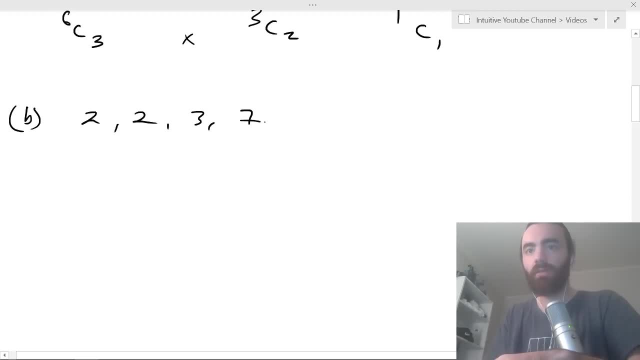 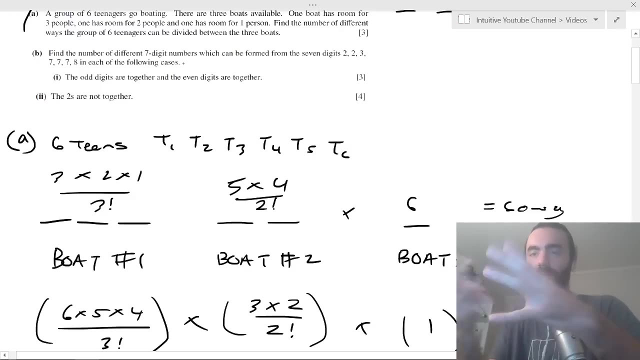 digit numbers which can be formed from the seven digits: two, two, three, seven, seven, seven, eight, okay, um, so we want to know how many ways we can form different digits or arrange these numbers with certain limitations, and these limitations are for the first cases, for i is that the odd. 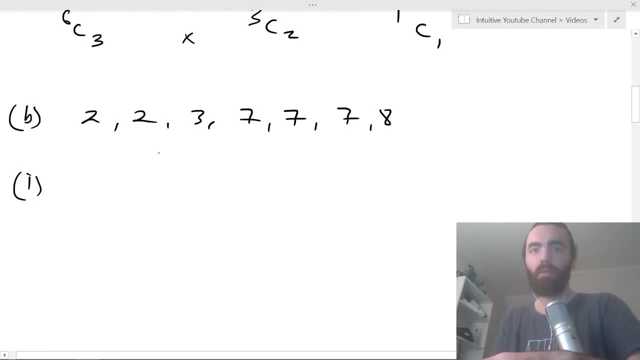 digits are together and the even digits are together. okay, so that means that all of the odd digits, the three, seven, seven, seven, that's together, and this is how i like to think about it. we put them in like a one slot or one box. all right, this is like one slot. 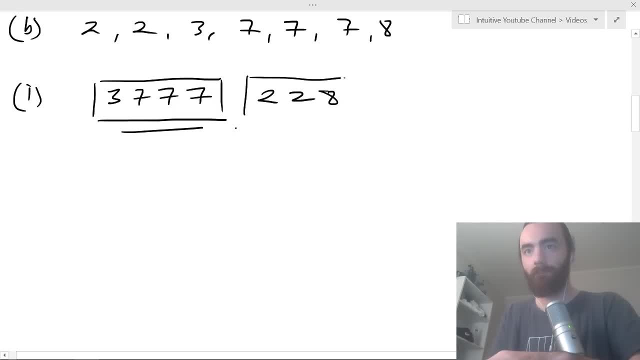 and then our second slot would be two, two, eight. okay, so then we can move these around two ways, right? so we can this three, three, i mean this three, seven, seven, seven could be in the first or the second, so there's two different ways for us for me to arrange that. so two times, well, how many ways? 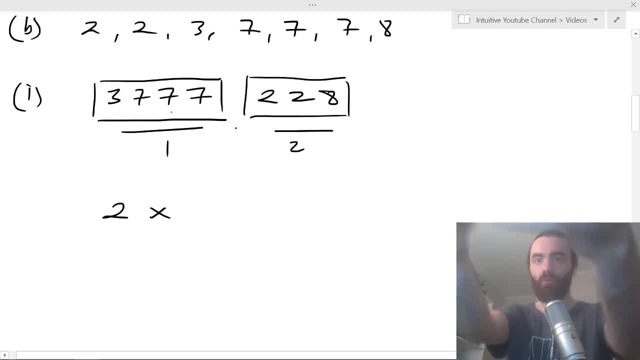 can i then arrange these, the internal structure of these boxes, the internal digits, right? so let's say for this one, well, there's four objects, so it'd be four factorial ways. but again we're over counting, because i'm, i'm, i'm counting the when i move these sevens. i'm saying that if we have three, three, seven as one, 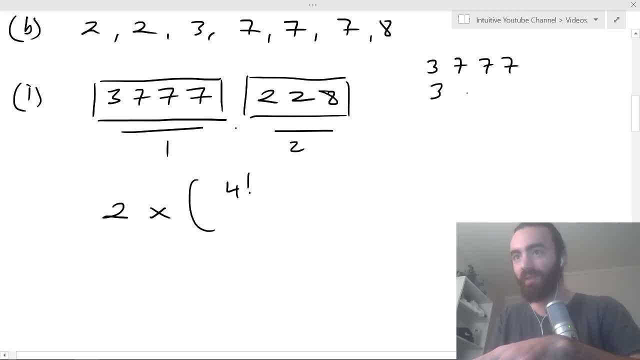 well, i'm also counting three and then i move these sevens around. so let's say i move this seven here, seven, seven, seven. but look, it's the same thing and i'm also counting when i move this seven with this seven, you know like. so i'm over counting, so i have to divide by the amount i'm over counting for each selection. 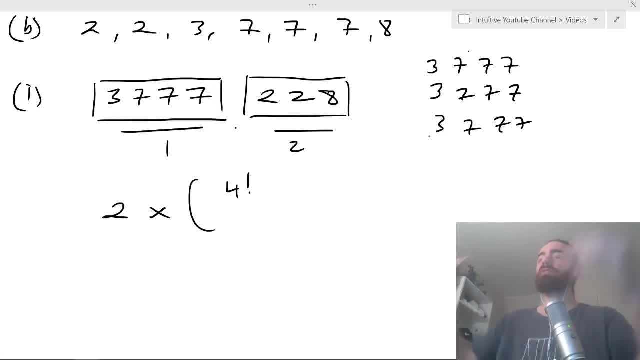 so for this, three, seven, seven, seven. i'm over counting three factorial ways, because there's three factorial ways for me to arrange these seven. so i need to divide by three factorial. okay, hope that makes sense, like, okay. and if i was to do seven, three, seven, seven, well, then again i'm. 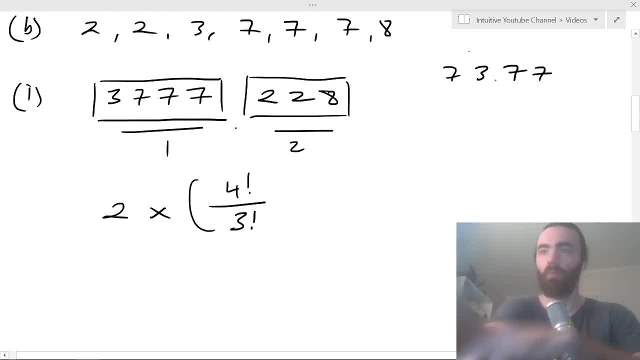 over counting. that's why i'm dividing, because for each, for this selection, i'm over counting. you know all the odds are together and then over counting, you know by three factorial that all the different ways i can arrange these three sevens, you know changing this one and 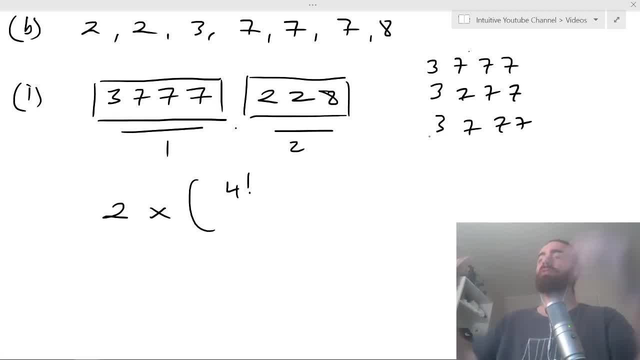 so for this, three, seven, seven, seven. i'm over counting three factorial ways because there's three factorial ways for me to arrange these seven, so i need to divide by three factorial. okay, i hope that makes sense. like okay, and if i was to do seven, three, seven, seven. 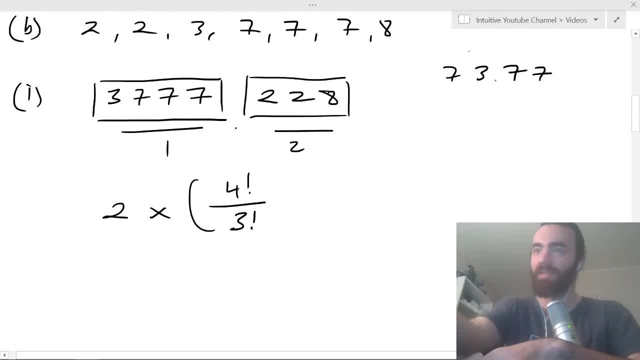 well, then again i'm over counting. that's why i'm dividing, because for each, for this selection, where you know all the odds are together, i'm then over counting. you know, by three factorial, that, all the different ways i can arrange these three sevens, you know changing this one and this one. 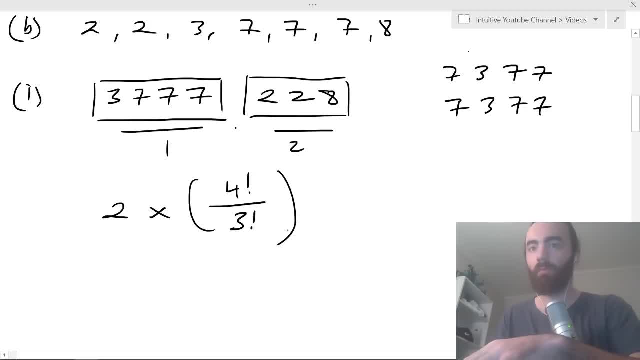 this one, this one, you know, they're all the same and they're all considered the same. so we divide by three factorial okay times this, which is going to be well, three factorial divided by, well, the number of ways i can arrange these twos, which is two factorial okay. 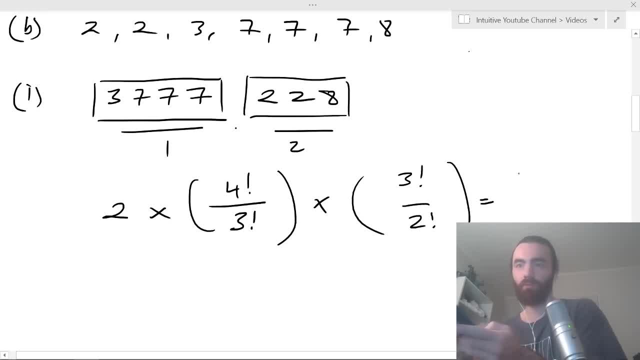 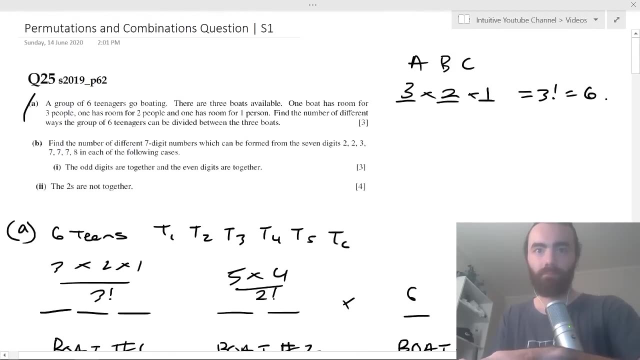 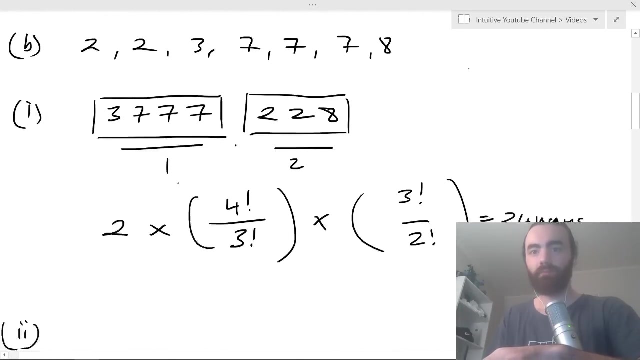 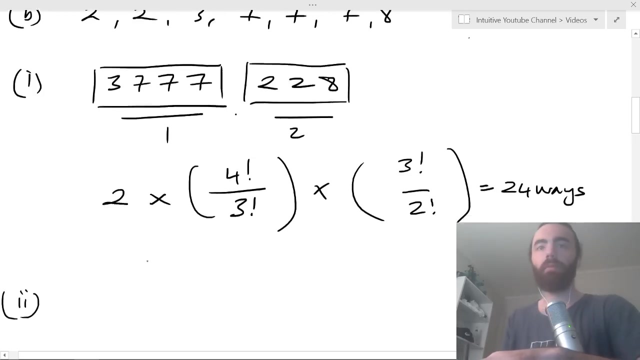 and that equals two or four. factorial will be four times three times two. so it's 24 ways. cool and again. so how many ways can we arrange these are objects if the twos are not together? well, the way i like to think about this is: is i like to think about slots between each one, because they do actually like to? 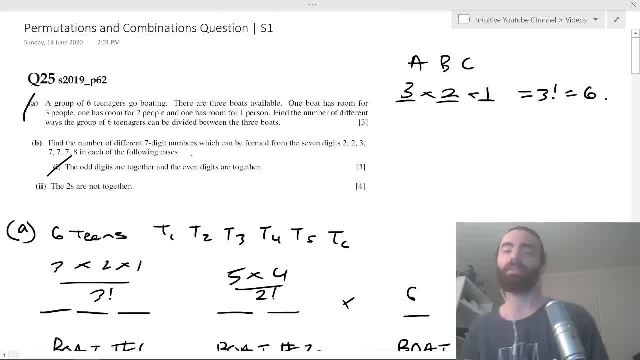 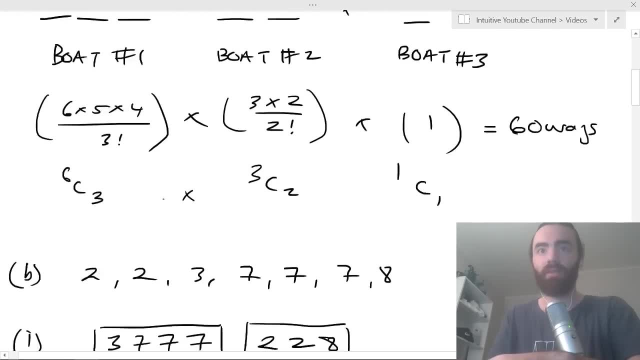 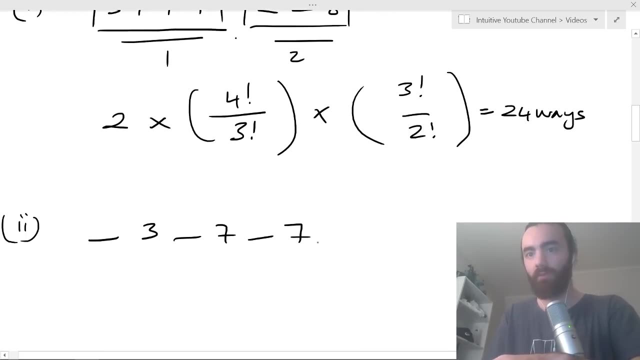 like, um, what they do actually like to ask this kind of question where two objects are never together in in the arrangements. so what i like to do for this is i'm going to say that, okay, i'm going to take the twos away first of all and say three, seven, seven, seven, eight, and you'll get when. 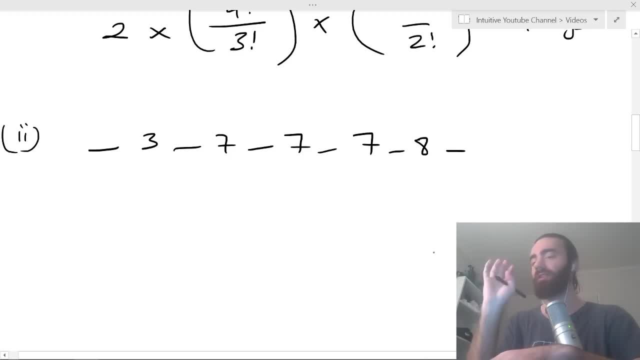 you start doing questions, you'll get your own way of doing each um style or whatever you want to call it. this is the way i like to do it. so then we have these twos here, and so let's say, if i put a two here and a two here, well then i'd form the um digit two, three, two, seven, seven, seven, eight, right. 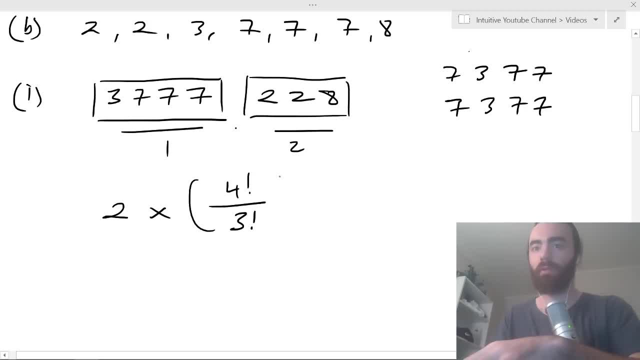 this one, this one, this one. you know, they're all the same and they're all considered the same. so we divide by three factorial okay times this, which is going to be, well, three factorial divided by well, the number of ways i can arrange these twos, which is two factorial okay. 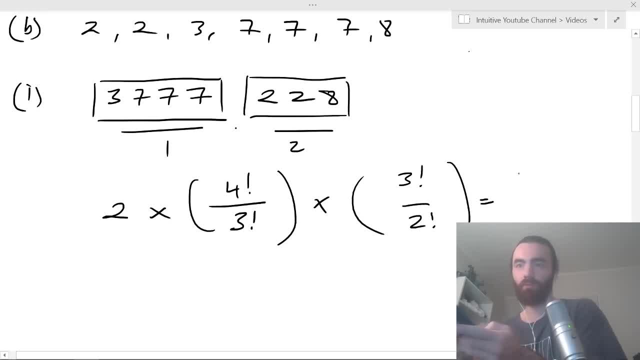 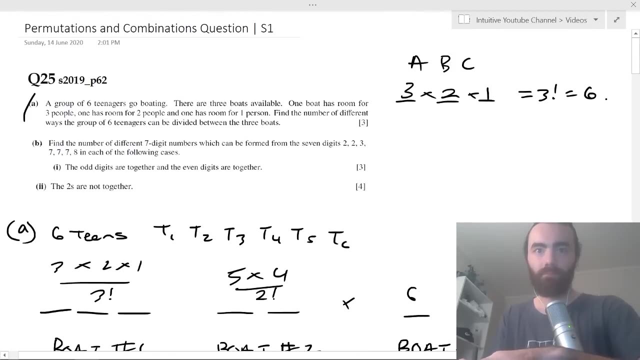 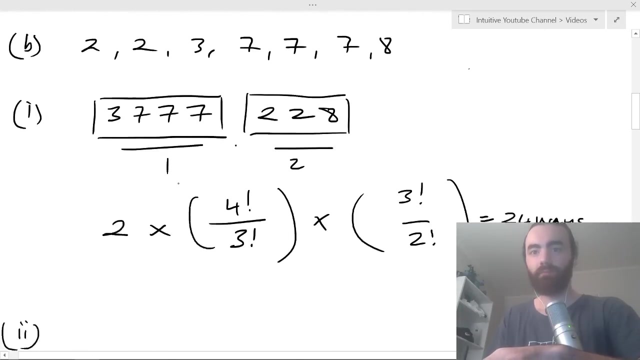 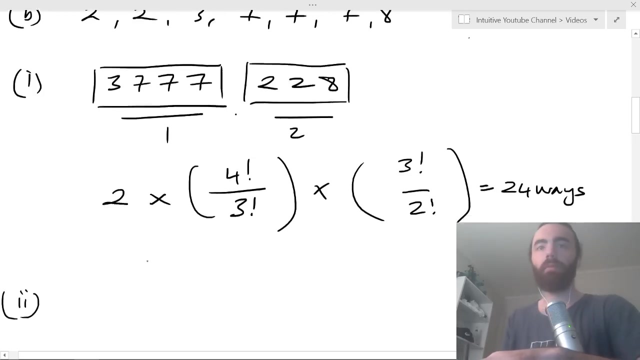 and that equals two or four. factorial will be four times three times two, so it's 24 ways. cool and again. so how many ways can we arrange these objects? um, if the twos are not together? well, the way i like to think about this is: is i like to think about slots between each one? because they do actually. 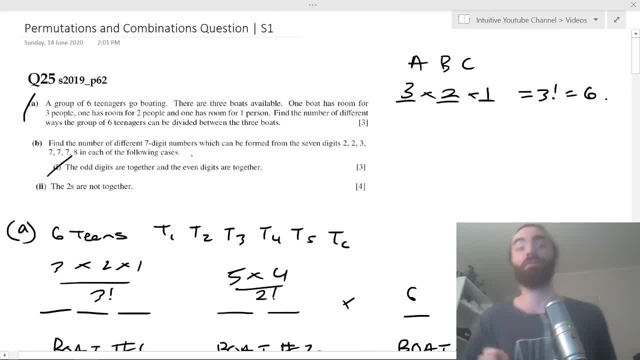 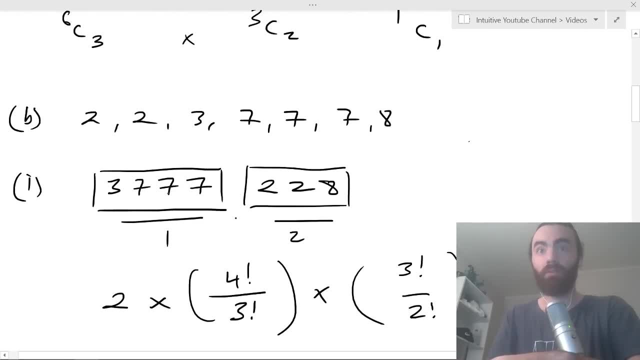 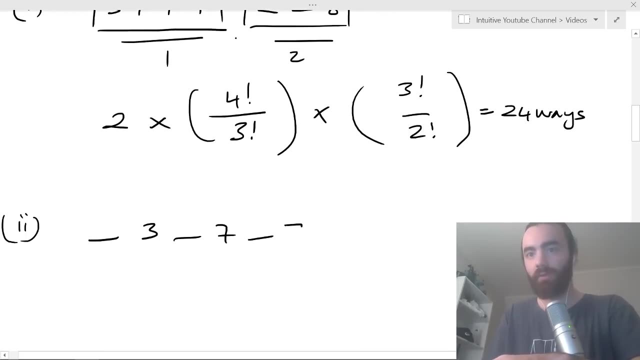 like to like, um, what they do actually like to ask this kind of question where two objects are never together in in the arrangements. so what i like to do for this is i'm gonna say that, okay, i'm gonna take the twos away first of all, and say three, seven, seven, seven. 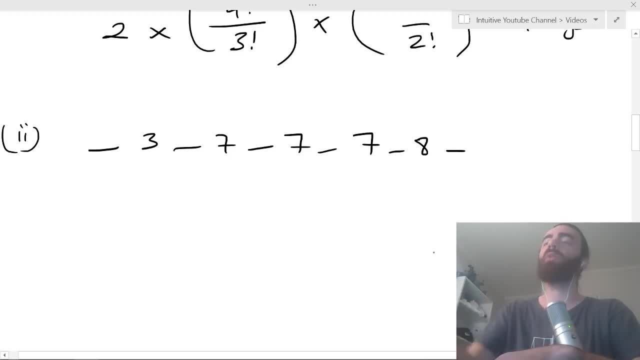 eight and you'll get, when you start doing questions, you'll get your own way of doing each um style or whatever you want to call it. this is the way i like to do it. so then we have these twos here, and so let's say, if i put a two here and a two here, well then i'd. 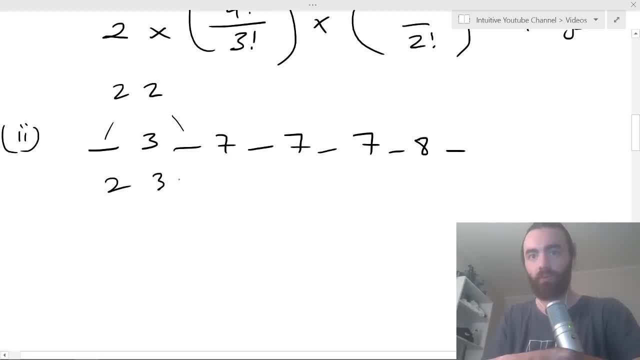 form the um digit: two, three, two, seven, seven, seven, eight, right. so i need to figure out how many ways i can do this. well, first of all, i'm going to figure out well, how many ways can i put twos, these two twos, into one. two, three, four, five, six slots. 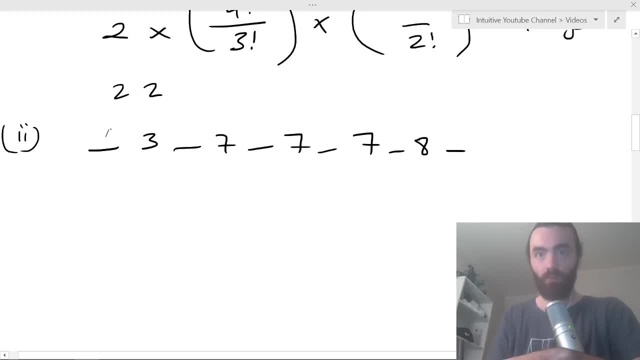 right. so the the way i can think about that is: well, there's one, two, three, four, five, six, way, six different places. i can put the first two, so i can say six, so i could put it here, here, here, here, here, and once i put that in, there's then times, five different places. i can put the. 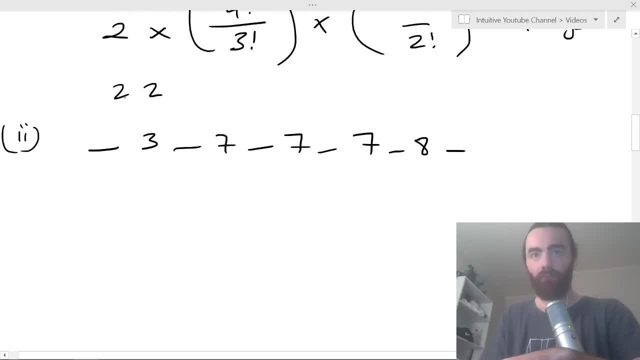 so i need to figure out how many ways i can do this. well, first of all, i'm going to figure out: well, how many ways can i put these twos, these two twos, into one two, three, four, five, six slots, right? so the way i can think about that is: well, there's one, two, three, four, five, six way, six different. 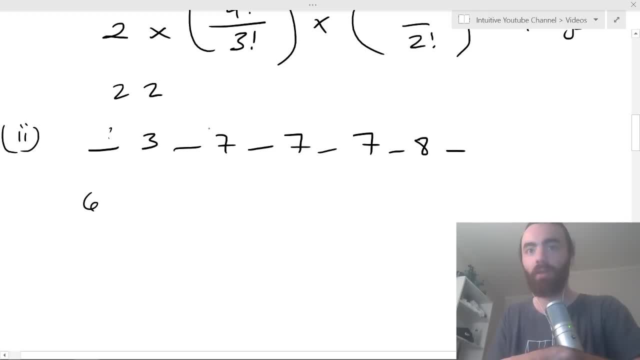 places. i can put the first two, so i can say six, so i could put it here, here, here, here, here, and once i put that in there's then times five different places. i can put the second two. but again we're over counting, because if i put a two there and a two there, 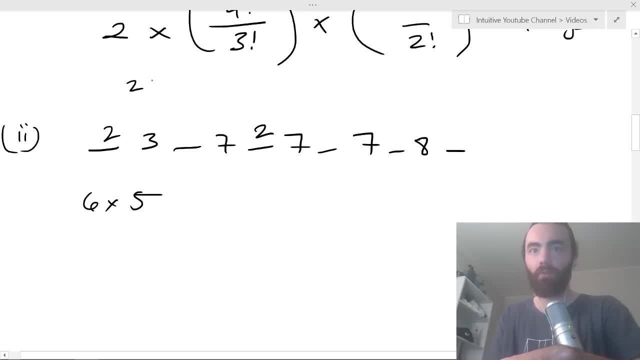 that's the same digit as if i put. so, let's say, if i put this first two here and the second two here, well, that's the same if i put the second two here and the first two here. so we have to divide by the number of ways we can arrange these twos, which is two factorial. so we've got this and then for that. 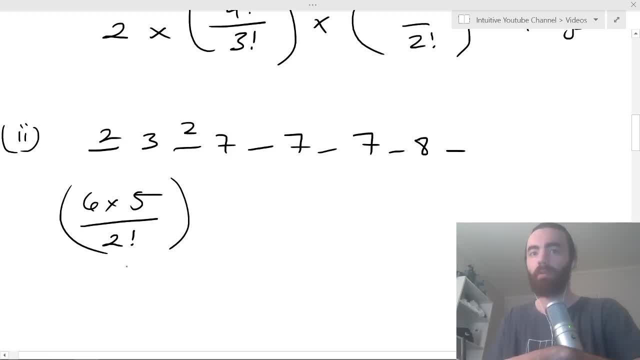 one thing let's say: if i put it here in, here for one of those, so one of these out of those, all of those different ways i can put the twos in where they're never together. i can then arrange these digits here, these one, two, three, four, five digits around those twos, so i can arrange those. 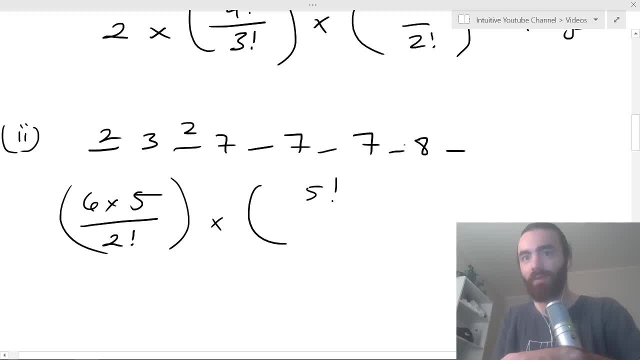 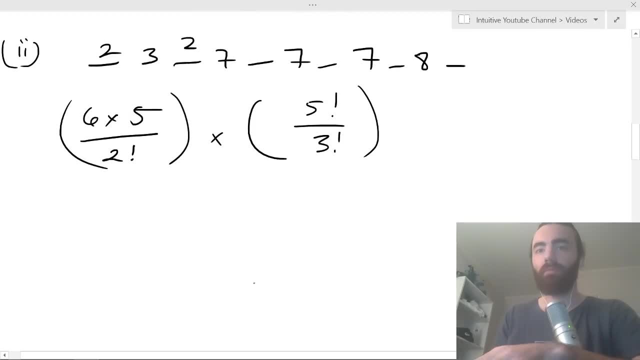 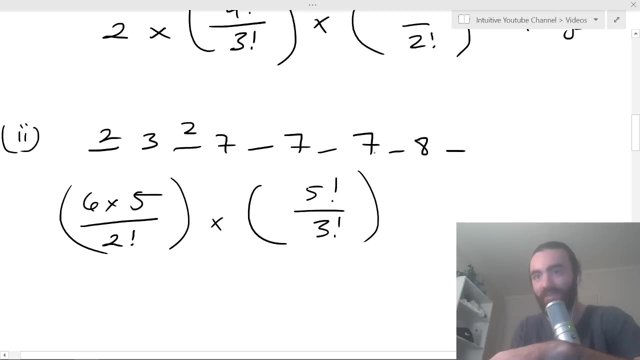 five digits times five factorial, different ways, divided by three factorial, because, remember, we're over counting again because of the sevens, right, does that make sense? so if i make this selection: two, three, two, seven, seven, seven, eight, i can then say: well, there's this many ways. 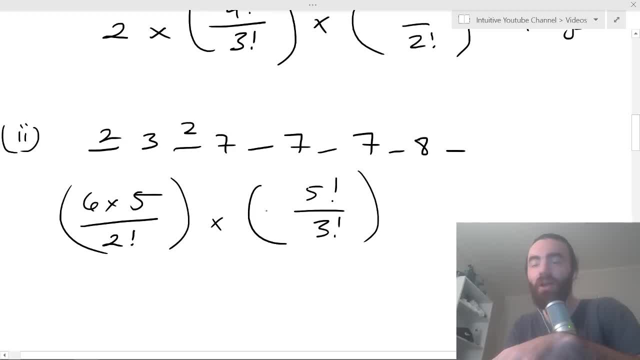 there's this many ways for me to put these twos in these slots and then times. there's this many ways for me to then arrange those remaining numbers around those twos? makes sense to me, i hope it makes sense to you, but if it doesn't, just ask in the comments and 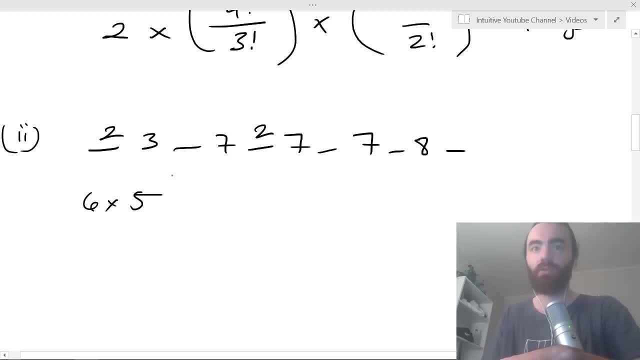 second two. but again we're over counting, because if i put a two there and a two there, well that's the same digit as if i put. so, let's say, if i put this first two here and the second two here, well that's the same if i put the second two here and the first two here. so we have to divide by the. 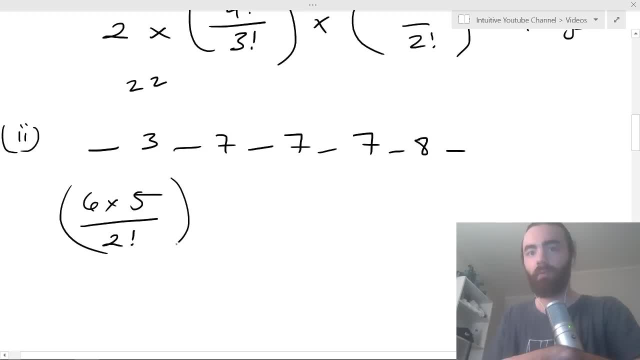 number of ways we can arrange these twos, which is two factorial. so we've got this, and then for that one thing, let's say, if i put it here and here for one of those, so one of these out of those, all of those different ways i can put the twos in where they're never together. i can then arrange these. 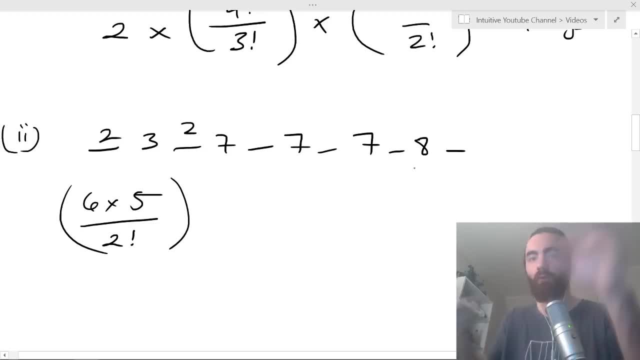 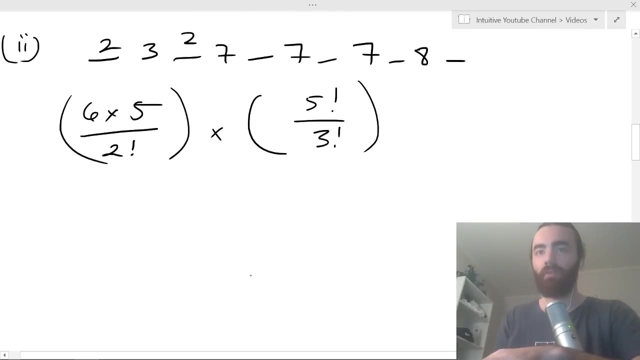 here these one, two, three, four, five digits around those twos, so i can arrange those five digits times five factorial, different ways, divided by three factorial, because remember, we're over counting again because of the sevens right. does that make sense? so if i make this selection two, 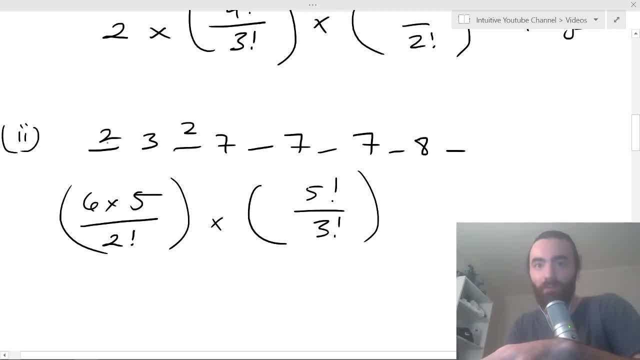 three, two, seven, seven, seven, eight. i can then say: well, there's this many ways, there's this many ways to put these twos in these slots and then times, there's this in many ways for me to then arrange those remaining numbers around those twos. it makes sense to me. i hope it makes sense to you. 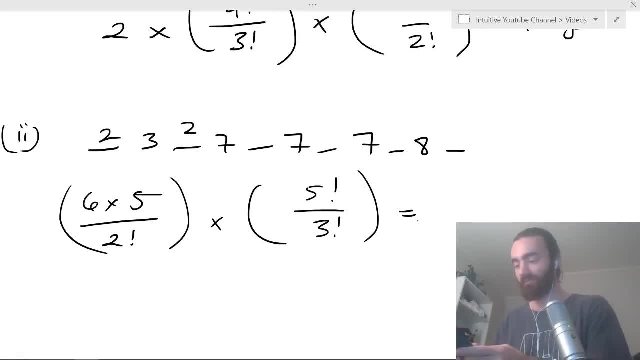 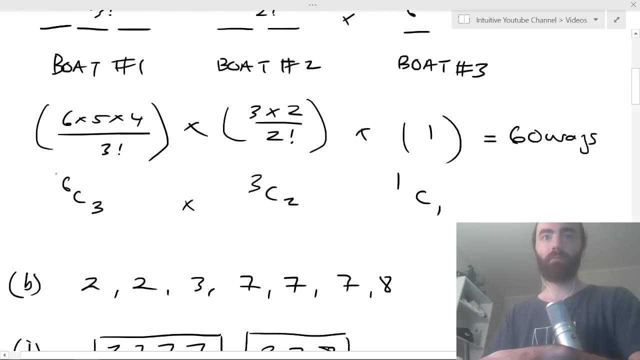 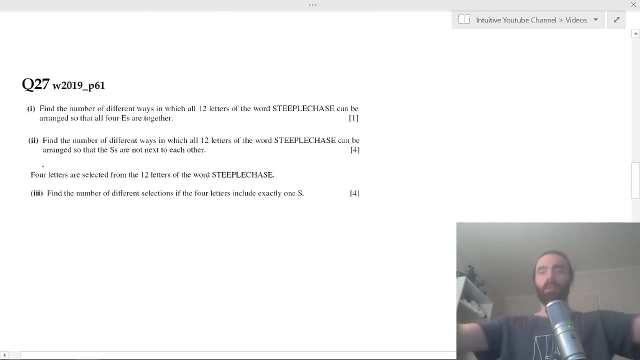 but if it doesn't, just ask in the comments, and i'll try to explain that better. so you put that in and you get times. five factorial divided by three factorial, this is 300 ways. cool, okay, so let's do another one. and they really like to ask this as well. so we've got sort of 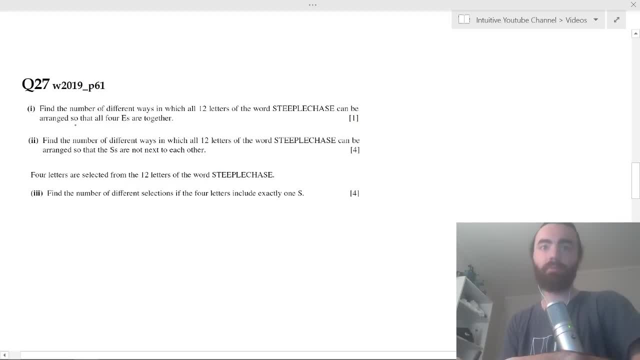 that first one, and then we've got this other one from again 2019.. so, okay, let's do this. so i find the number of different ways in which 12 letters of this word can be arranged so that all four e's are together okay. so let's write this out. 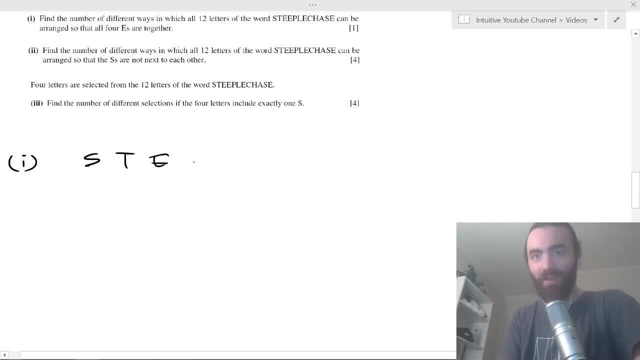 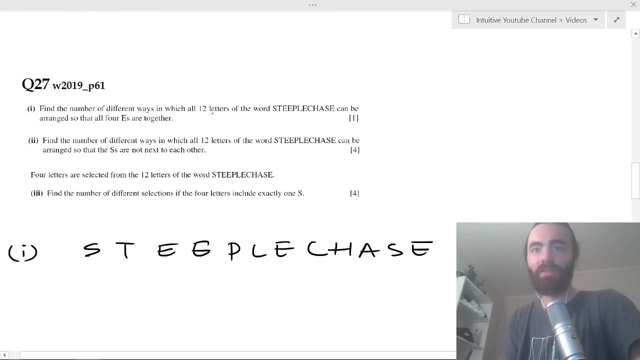 s? what is it? steeple case? okay, see what i mean. it's just so random. steeple, oh, steeple chase- could have been a disaster. okay, so we've got this random as word, which i don't even know what it is: steeple chase, um. so how many different ways can we? 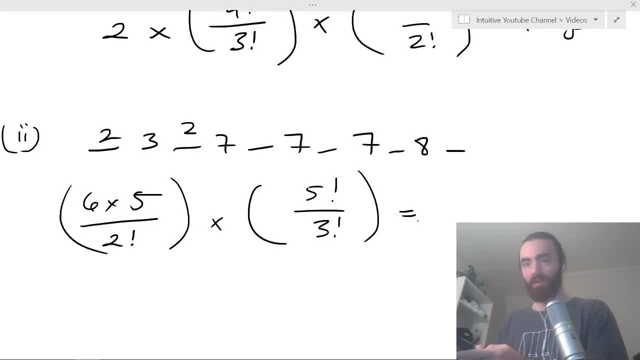 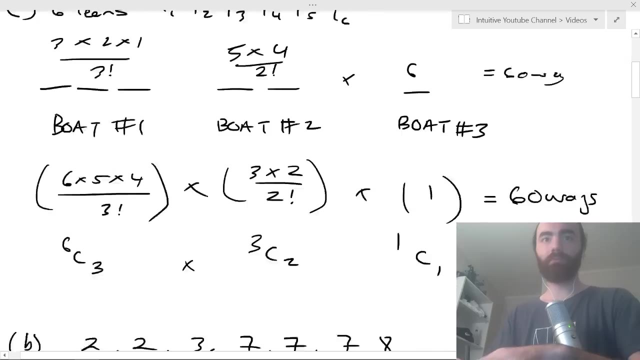 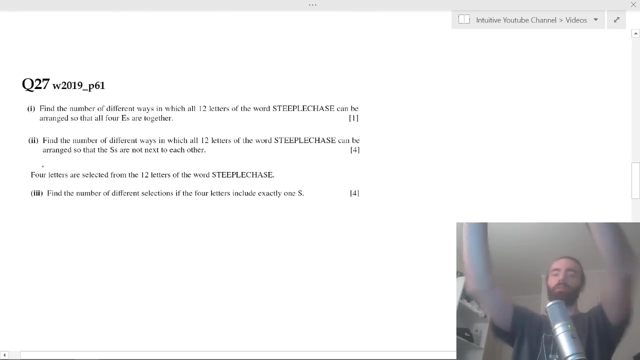 i'm trying to explain that better. so you put that in and you get times: five factorial divided by three factorial, this is 300 ways. cool, okay. so let's do another one, and i really like to ask this as well: so we've got sort of that first one and then we've got this other one from again 2019. 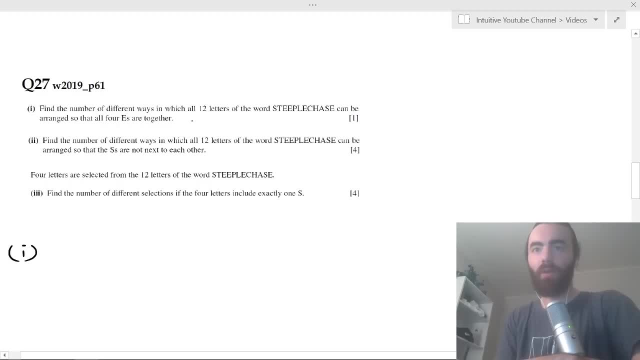 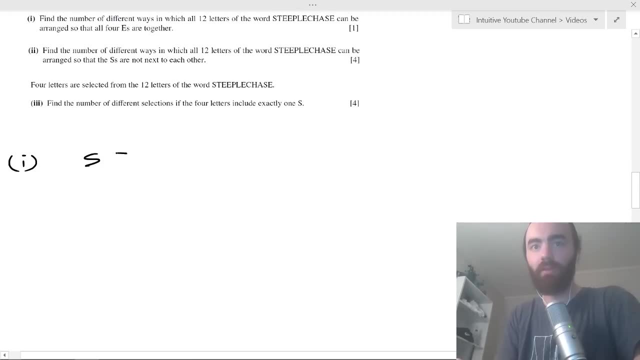 so, okay, let's do this. so i find the number of different ways in which 12 letters of this word can be arranged so that all four e's are together okay, so let's write this out: s, what is it? steeple case. okay, see what i mean, just like. 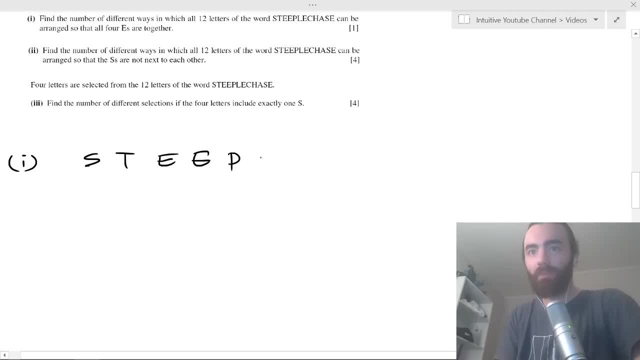 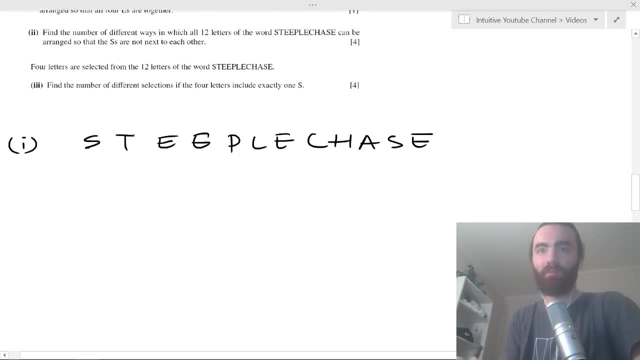 so random steeple. oh, steeplechase could have been a disaster. okay, so we've got this random as word, which i don't even know what it is: steeplechase. um. so how many different ways can we arrange these 12 letters so that all four e's are together? well, 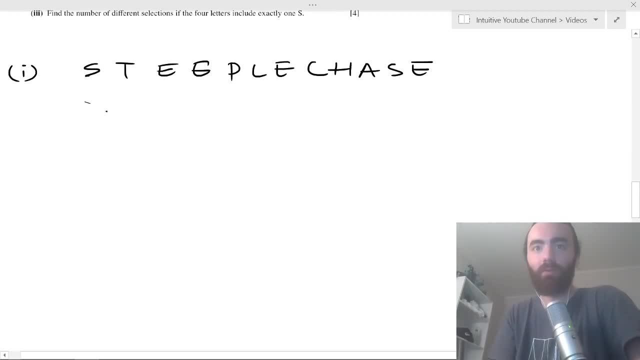 it's similar to the thing before, where i grouped all the odds and evens. well, okay, we've got these e's- two, three, four- in this one slot, and then we've got the remainder, which is the the s, t, p, l, c, h, a, s. i need to be careful. so we've got four, five, six, seven, eight, nine, ten, eleven, twelve. so 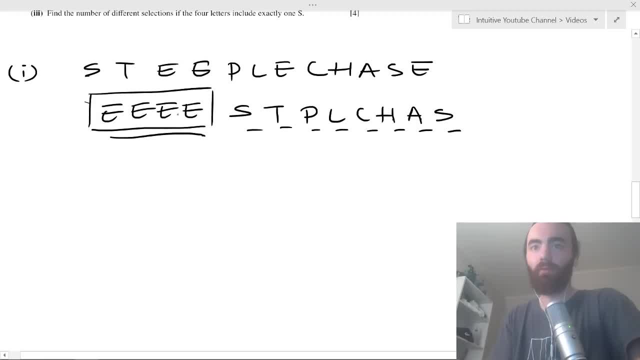 we've got these, okay. so how many ways can i arrange this? well, there's one plus eight, so there's nine slots. so i can arrange that nine factorial ways, right, and that will keep the e's together. and then- but i have to be careful here, because i've got these two- 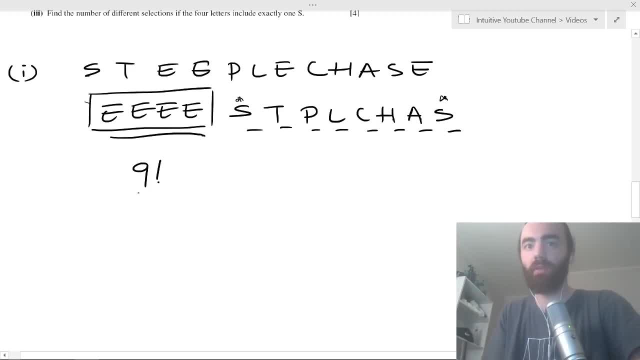 s's. so again, i'm over counting when i'm switching these two s's. so we have to divide by the number of ways that we can arrange those two s's, which is two factorial. okay, that's all the ways. you know, if we had more double ups, then we'd have to divide by more stuff, but we don't, so it's. 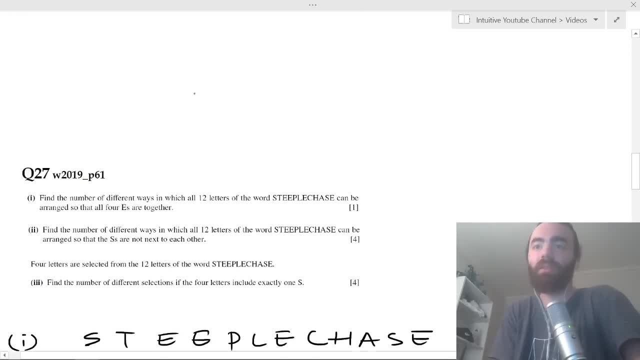 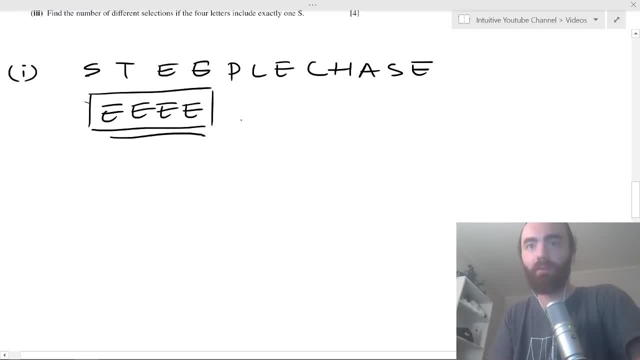 in this one slot, and then we've got the remainder, which is that the S T, P, L, C H A S. I need to be careful with this. so we've got 4,, 5,, 6,, 7,, 8,, 9,, 10,, 11,, 12. 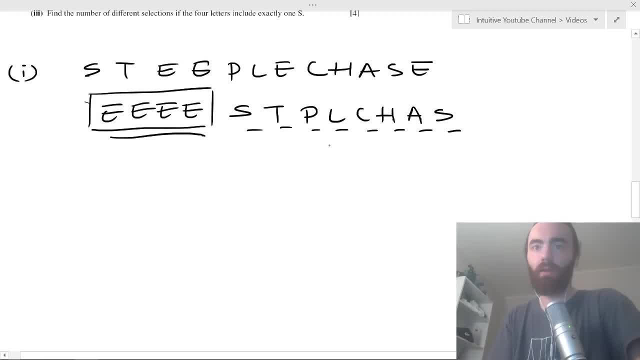 so we've got these okay. so how many ways can I arrange this? well, there's 1 plus 8, so there's nine slots. so I can arrange that nine factorial ways, right, and that will keep the E's together. but I have to be careful here, because I've got these two S's. 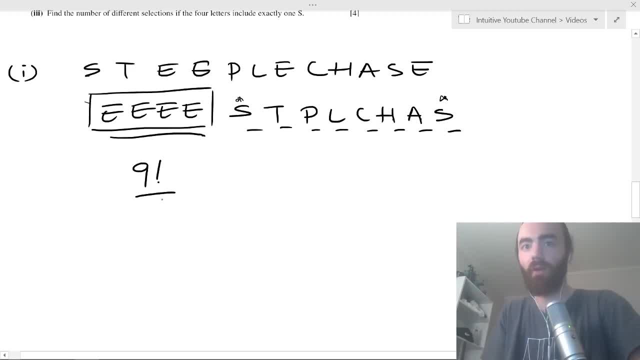 so again I'm over counting when I'm switching these two S's. so we have to divide by the number of ways that we can arrange those two S's, which is 2 factorial. that's all the ways, and if we had more double ups then we'd have to divide. 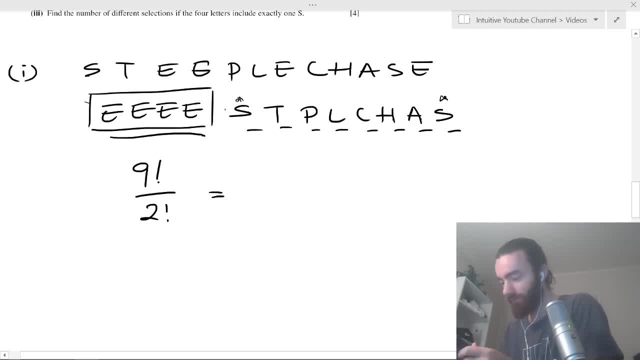 by more stuff, but we don't. so it's 9 factorial divided by 2 factorial, which is 1000. nah, it's a lot of ways: 11444, Do it your way: 1400 ways, so 181440 ways. cool tick. 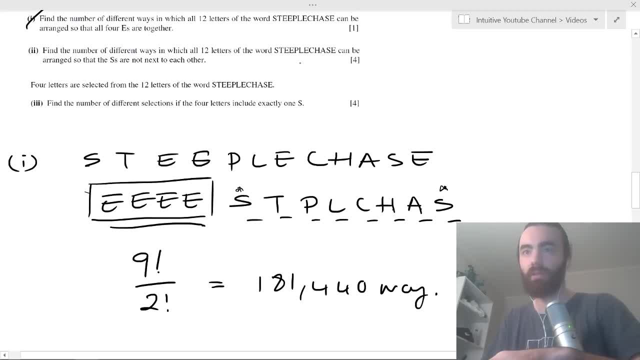 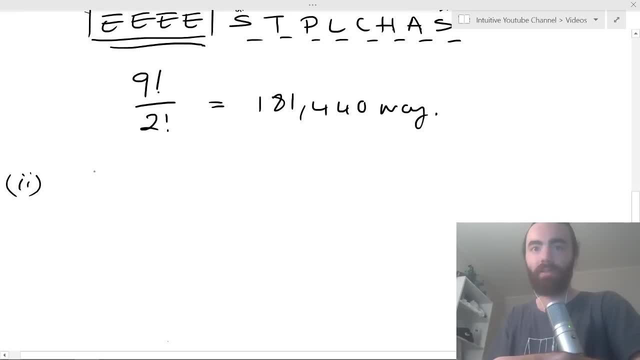 find the number of different ways in which all twelve letters of the word steeplechase can arrange so that the S's are not next to each other. well, look, this is the same as the other thing, right, okay, so let's take those S's out. 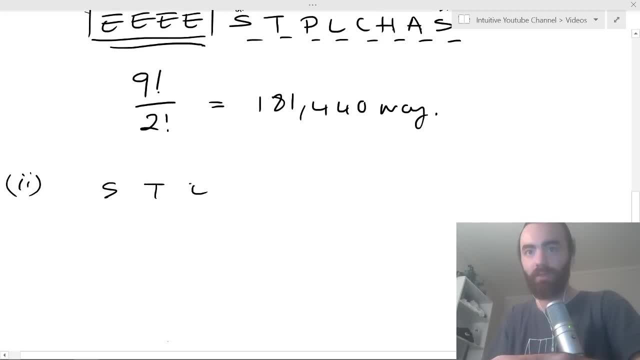 and we get. so let's write it down, our letter at the top. we've got 30 pi to triplesimiz our letter: s? t e p? l? e, steeple chay one, two, three, four, five, six, seven, eight, nine, ten, eleven, twelve, cool, okay. so let's take these s's out and again, let's do the same thing that i did before. 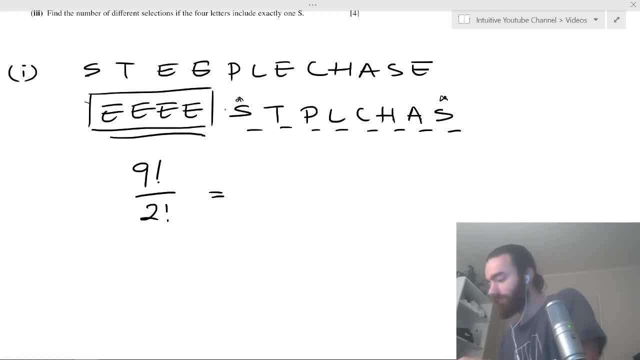 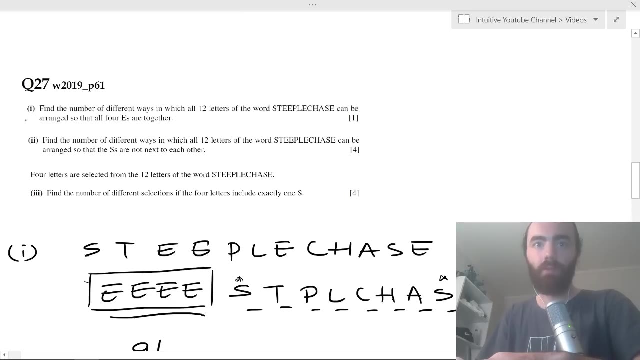 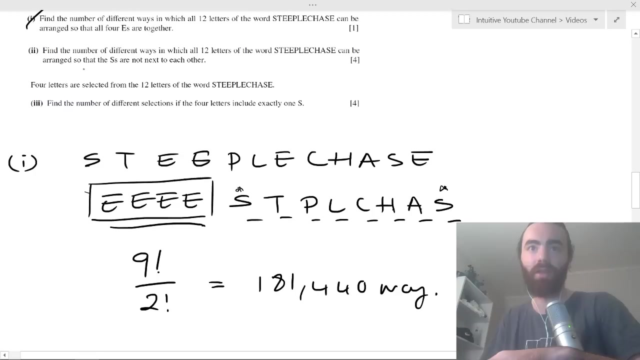 nine factorial divided by two factorial, which is one thousand. damn, it's a lot of ways. one thousand one hundred 440 ways, so 181 440 ways. cool tick, find the number of different ways in which all 12 letters of the word steeplechase can be arranged so that the s's are not next to each other. well, look this. 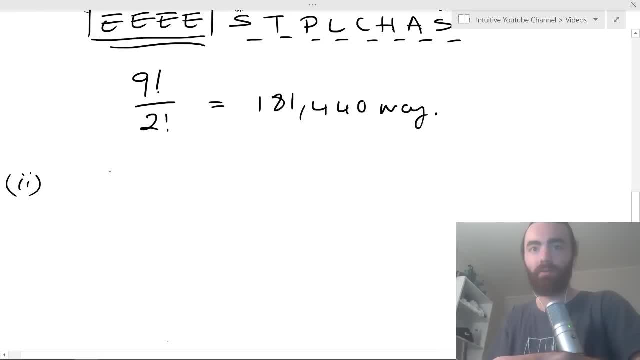 is the same as the other thing, right, okay, so let's take those s's out and we get. so let's right out our letter. ste steeple je 5 slots for two s e, z, another e, o, d, e, an, e, p, u, p e. 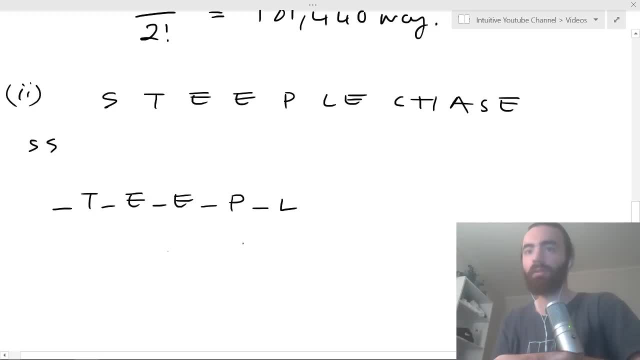 x and L. I like to draw it out because it's good for me. I like to visualize it. what's going on? I want to know what's going on here. C, H and A and E, so we should have 10 here. 1, 2, 5, 6, 7, 8, 9, 10, cool. so how many different ways can I put these two S's into these? 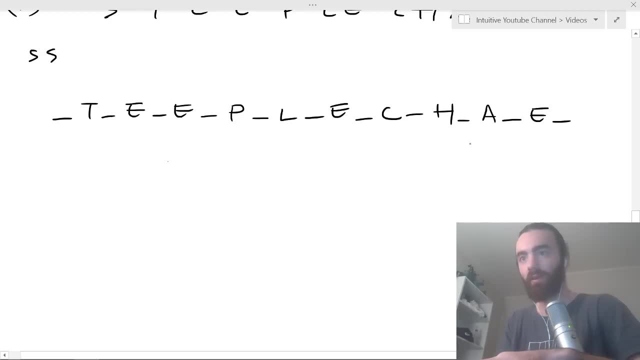 1, 2, 3, 4, 5, 6, 7, 8, 9, 10, 11 slots. again, there's 11 different ways for the first S, times 10 different, because then one of the slots is taken. 10 different ways for the second S, but then again. 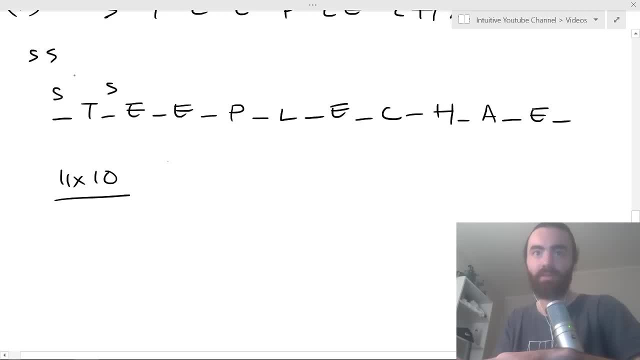 remember, we have to take into account- you know we're over counting- S S, first S, second S. that's the same as second S, first S. you know, if we were to label them, it's the same arrangement of letters. okay, so we divide by two factorial, and then we have to times by. well, how many ways can we? 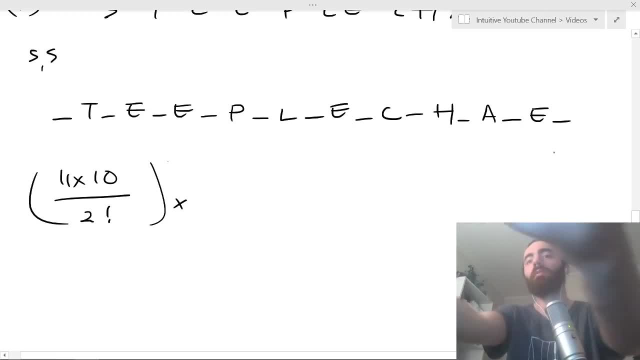 arrange these. then, once we made the selection, the times by how many ways that we can arrange these letters around those S's, and I sort of went through that before. so this is going to be well, we have 10, right, we have 10 letters, so 10 factorial, but then we have these four E's. so 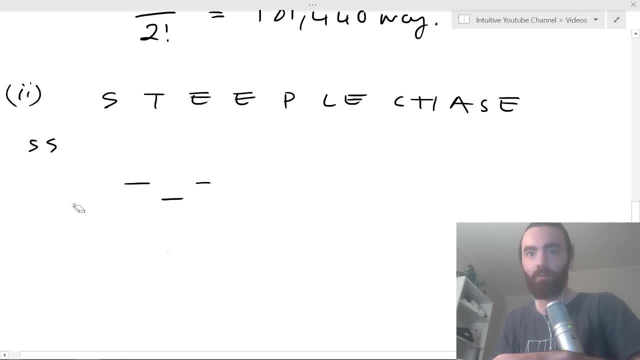 so we've got these slots, then we've got a t, an, e. i might need more space. we're gonna have a t and e, another e, a p and l. i like to draw it out because it's good for me. i like to visualize it. what's going on? you know, i want to know what's going on here- c a, h and a and e, so we should. 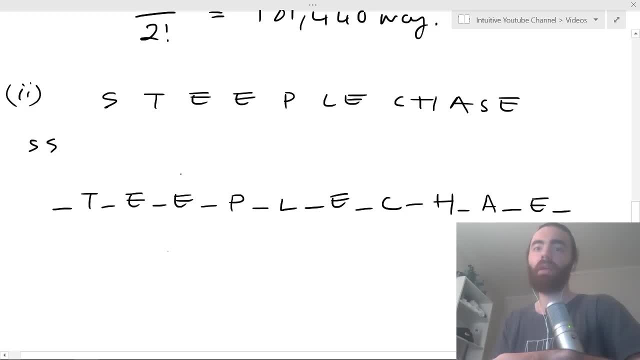 have ten here: one, two, three, four, five, six, seven, eight, nine, ten, cool. so how many different ways can i put these two s's into these? one, two, three, four, five, six, seven, eight, nine, ten, eleven slots. there's again. there's eleven different ways. for the first s times, ten. 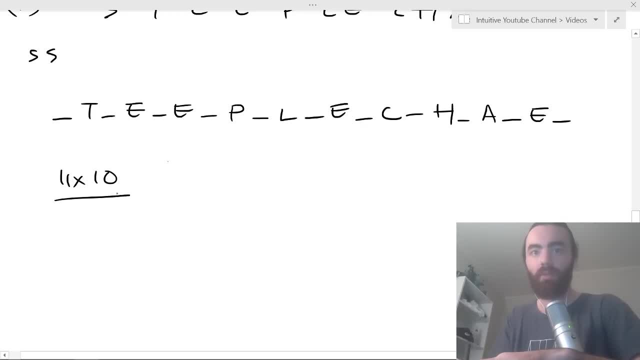 different, because then one of the slots is taken ten different ways. for the second s, but then again, remember, we have to take into account you know we're over counting s s first s second s, that's the same as second s first s. you know, if we were to label them, it's the same arrangement. 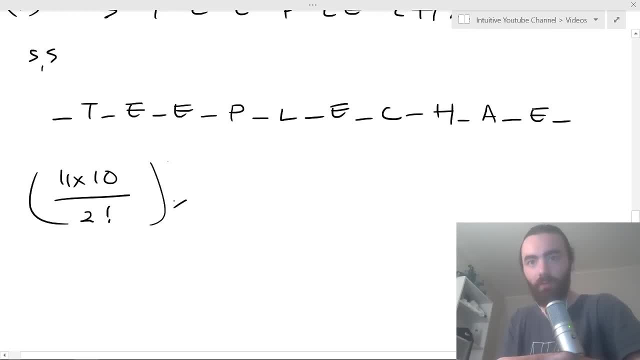 of letters. okay, so we divide by two factorial, and then we have to times by well, how many ways can we arrange these? then, once we made the selection, the times by how many ways that we can arrange these letters around those s's, and i sort of went through that before. so this is going to be. 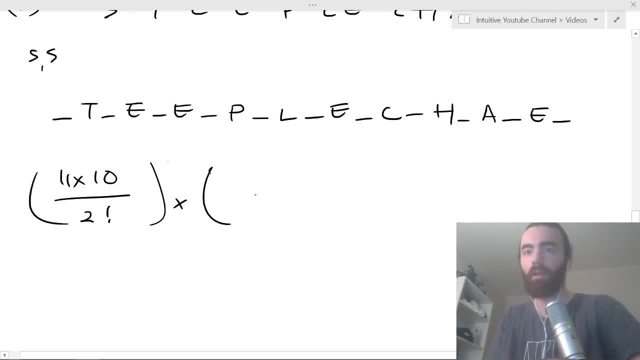 well, we have 10, right, we have 10 letters, so 10 factorial. but then we have these four e's. so then again we're over counting by for each one of those arrangements. we're over counting by four factorial. so we have to divide by four factorial- cool. and you chuck all that in to your calculator and you 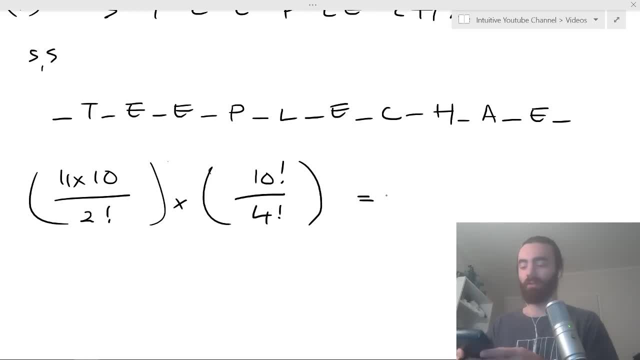 be you think, um the lords, that you don't have to calculate this yourself without this incredible device divided by four, factorial eight million, eight million three hundred and sixteen thousand. you know, it's actually really powerful like technique. if there's that many ways to arrange some letters, imagine how many arrangements of other things there are like. 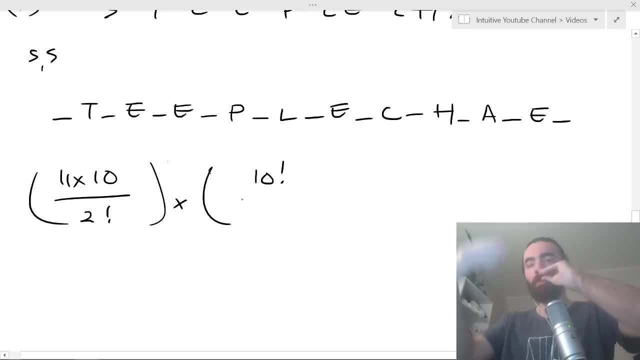 then again, we're over counting by for each one of those arrangements we're over counting by four factorial. so we have to divide by four factorial, cool, and you chuck all that in you to your calculator and you be you. thank um the lords that you don't have to calculate this. 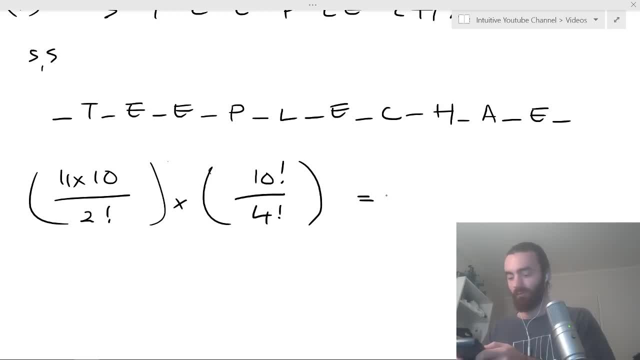 yourself without this incredible device divided by four factorial eight million, eight million three hundred and sixteen thousand, you know, um, it's actually really really powerful like technique. if there's that many ways to arrange some letters, imagine how many arrangements of other things there are, like particles or I don't know, human. 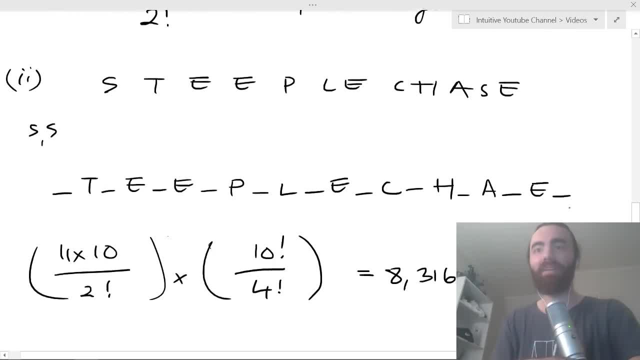 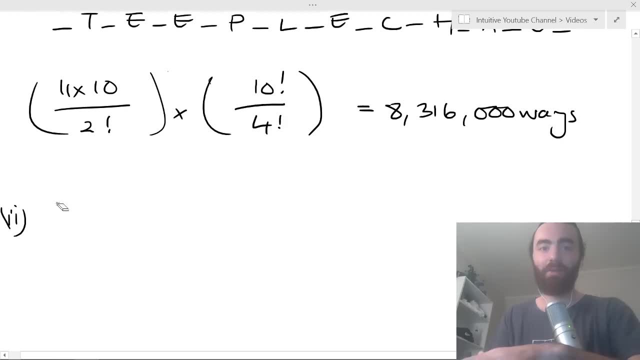 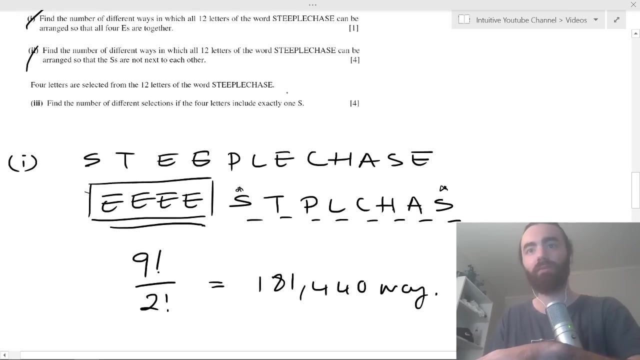 ideas. imagine how many different arrangements there are of that, if there's eight million of these stupid set of letters. anyway, that's hilarious. okay, oh, aye, aye, aye, okay, okay, okay, okay, okay, I'm hungry. okay, I'm hungry. okay, and the last one. so four letters are selected from these twelve letters of steeplechase. 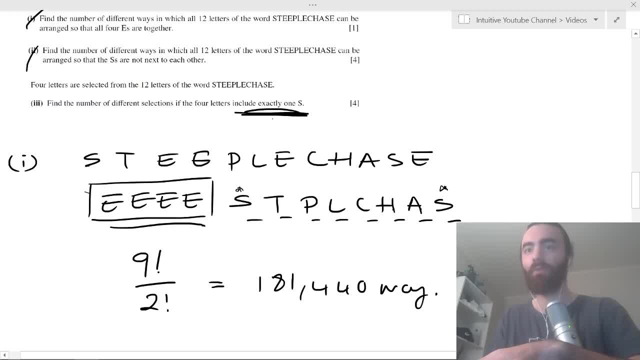 find the number of different selections of the four letters and include exactly one s. okay, so I'm going to write it out again: s-t-e-e-p-l-e steeplechase- 1, 2, 3, 4, 5, 6, 7, 8. 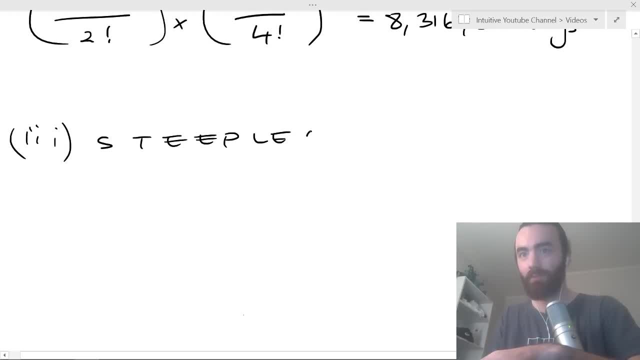 9, 10, 11 or 12 ". ok, so I can even MAJOR yourself later. okay, alright, then we're gonna pop the sake one over ALL men you've которой see, uh andantomash. yeah, thank you, You are таким. just can I cast here? 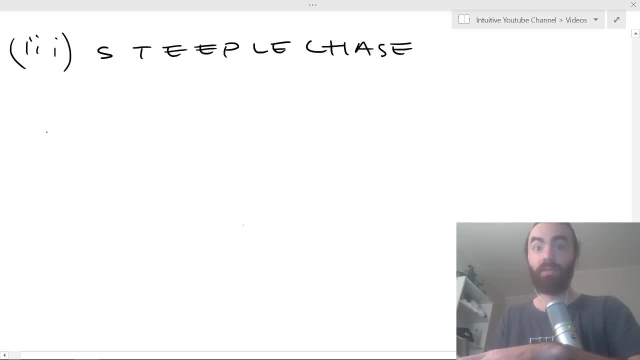 Erick, with the best one power. everything else within myself will do So, don't worry about it. of the letters is guaranteed to be an s. it's pretty much like we're only selecting. there's only one way to do that right: it's going to be an s, so one of them is guaranteed to be an s. 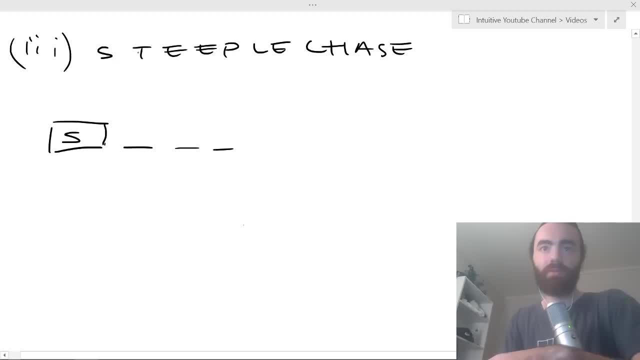 and then the remaining ones. well, they're up for grabs. so we've got the remaining letters, which is t, e, e, p, l, e, c, h, a, e. so you've got one, two, three, four, five, six, seven, eight, nine, ten. cool, so you got ten letters. now you might think it okay. well, then we've got ten letters. so then there's just. 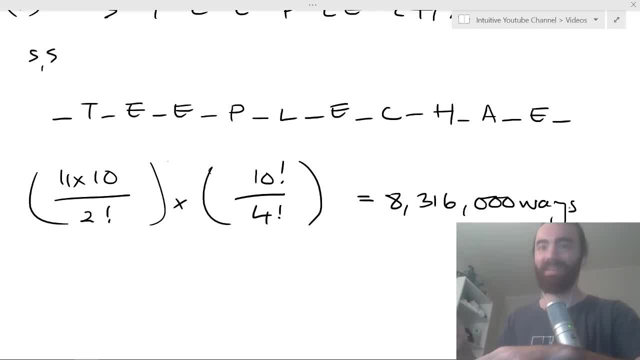 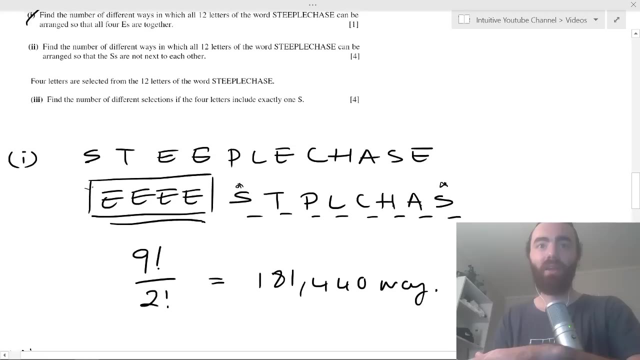 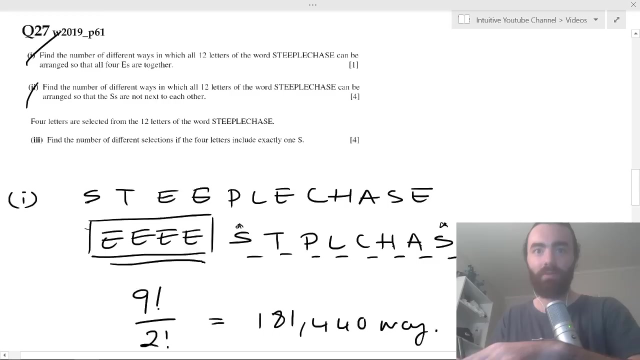 particles or, i don't know, human ideas. imagine how many different arrangements there are of that if there's a million of these stupid set of letters. anyway, that's hilarious. okay, oh, i'm hungry. last one, so four letters are selected from these 12 letters of steeplechase. find the number of. 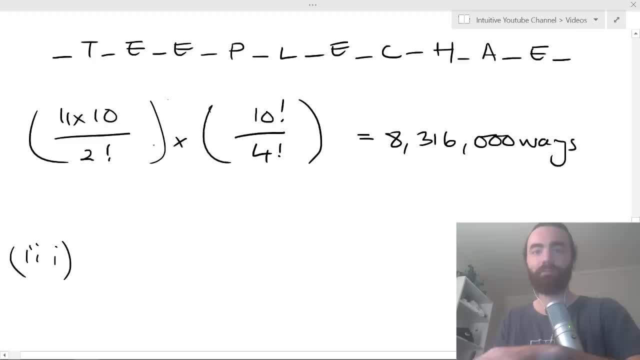 different selections and the four letters include exactly one s. okay, so i'm going to write it out again: s-t-e-e-p-l-e. steeplechase one, two, three, four, five, six, seven, eight, nine, ten, twelve, cool, and we're supposed to select four letters, but one of the letters is guaranteed to be an s. it's pretty. 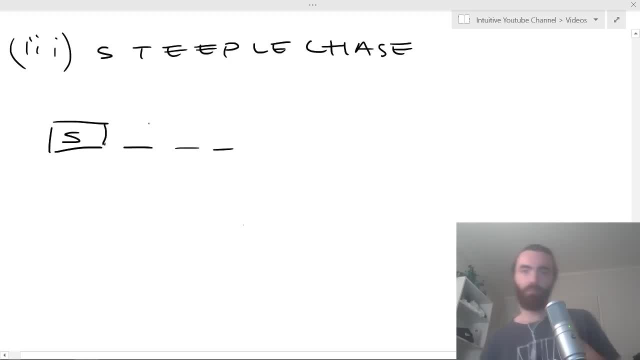 much like we only select. there's only one way to do that right. it's going to be an s, so one of them is guaranteed to be an s, and then the remaining ones. well, they're up for grabs. so we've got the remaining letters, which is t-e-e-p-l-e-c-h-a-e. so you've got one, two, three, four, five, six, seven. 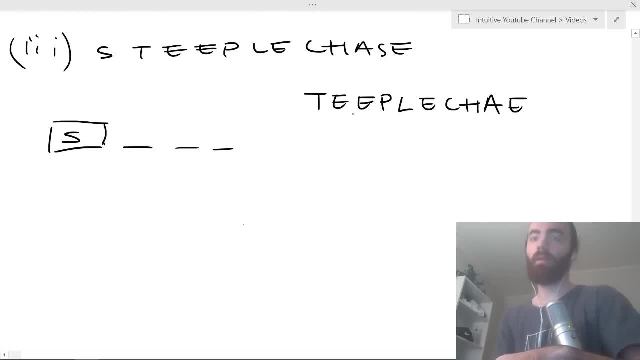 eight, nine, ten, cool, so you've got ten letters. now you might think it: okay, well, then we're going to do that again. we've got ten letters. so then there's just ten times nine times eight, right different ways to put these letters in. then we just divide by three, factorial, but actually you've 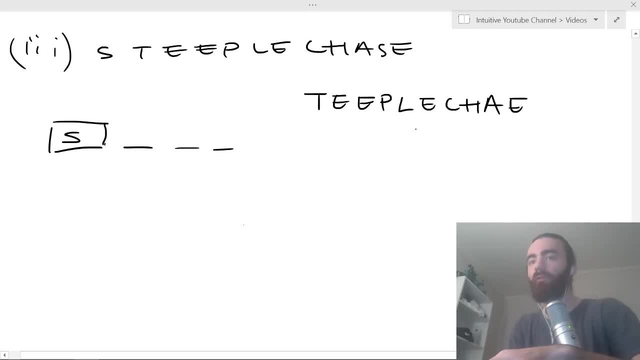 got to be careful because, look, you've got e's, you've got four e's here. so when you make a selection for the e's, we're over counting. again, it's this idea of over counting. we're over counting because, you know, for, let's say, selecting this e, there's one, two, three, like if we were to name these. 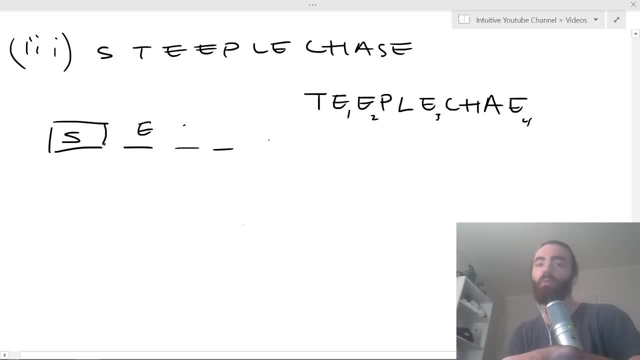 e's differently. there's four different ways that we can do that where. but they're all creating the same selection, so we're over counting the e. so we need to take the e's into account and each. so when we select no e's, when we select one e, when we select two e, when we select three e's, we need to take those. 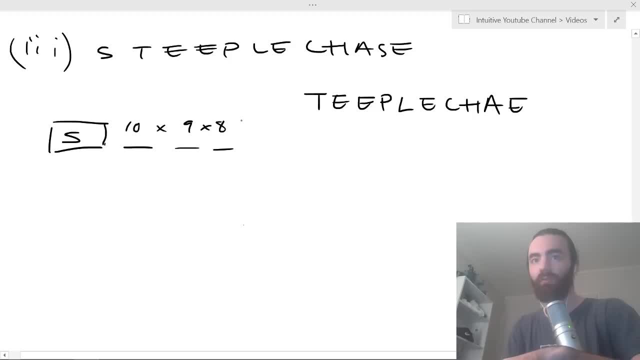 ten times, nine times, eight, right different ways to put these letters in. then we just divide by three: factorial. but actually you've got to be careful because look, you've got ease, you've got four easier. so when you make a selection for the ease, we're over counting again, this idea of over. 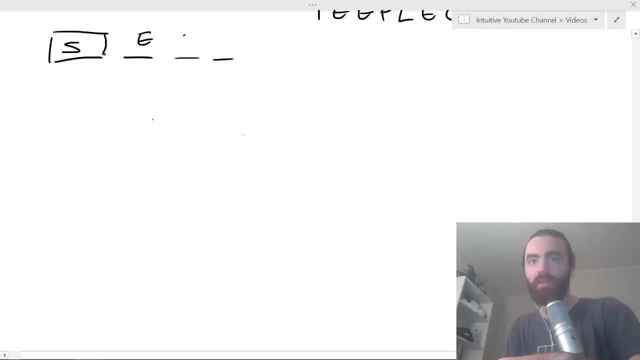 counting or over counting, because, you know, for, let's say, selecting this e, there's one, two, three, like if we were to name these letters, and then we just divide them by three and then we just divide these e's differently. there's one, two, three, four different ways that we can do that where. but 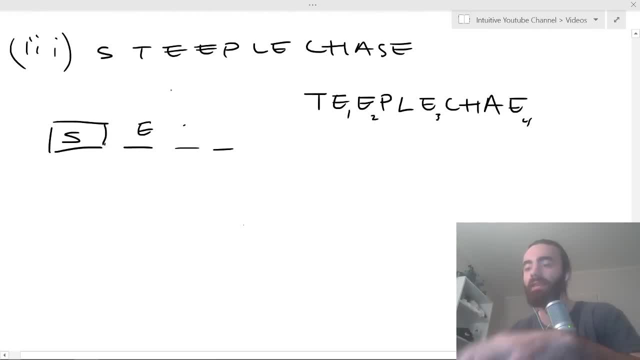 they're all creating the same selection, so we're over counting the e. so we need to take the ease into account, and each. so when we select no ease, when we select one e, when we select two e, when we select three e's, we need to take those into account. so, taking away the ease and just thinking, 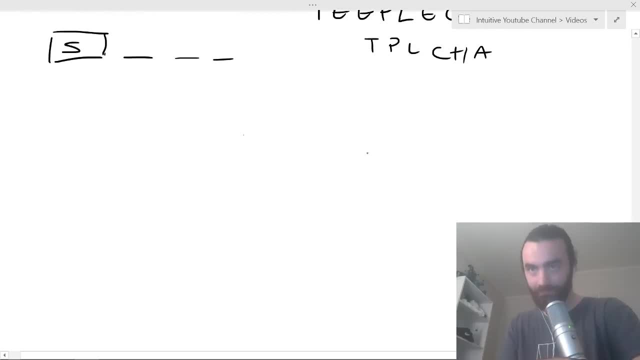 about the final letters that we have: t, p, l, c, h, a. so let's take the case where we've got zero ease, right, so we've got zero ease. well then, there's from this, from the remaining letters, we've got one, two, three, four, five, six, so there's six different. 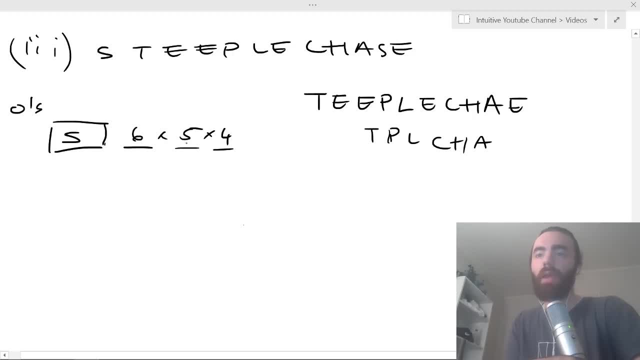 ways times, and then five different ways times in four different ways. and remember, if we let's say tpl, we calculate tpl. i mean pick tpl. well, this is the same as lpt, which is the same as you know. it's the same thing. so then we have to divide by three, factorial, and then we have to divide by three. 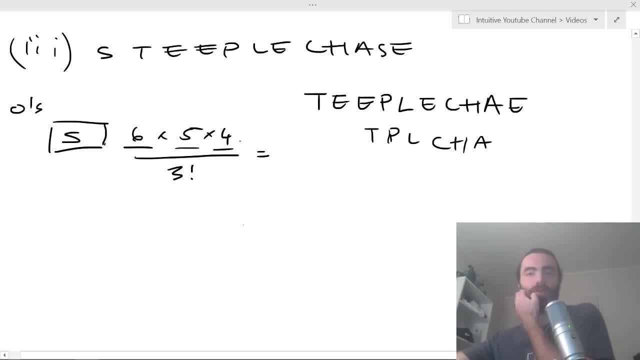 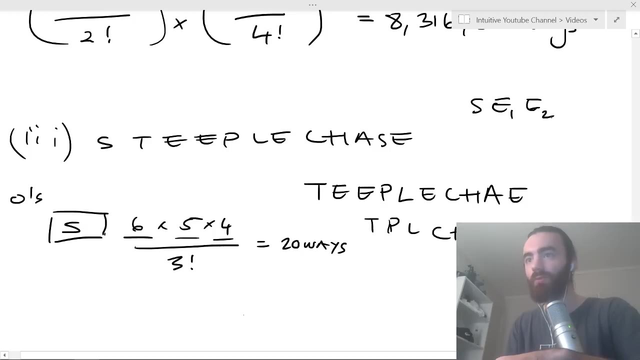 factorial that equals. so for zero ease there's no easepick. you know, six times five times four divided by three factorial. so there's 20 ways to do that and i hope it makes sense that why i'm taking out the ease, because look, if i pick s, e, 1 e, 2, t, like that's the same we're counting if 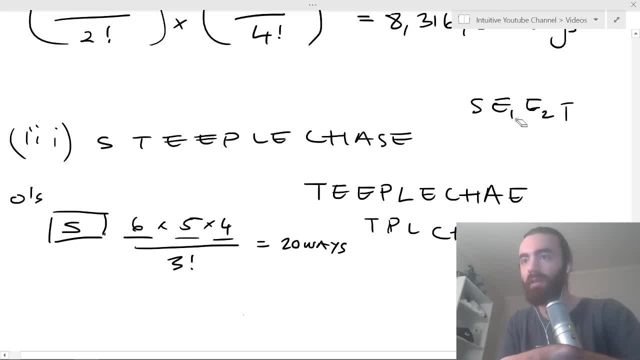 we were to do it like i said before, like with the 10 times nine. well then, we're also counting three, two. we're also counting four, two, like if these e's are different, four, three, we can. we're over counting by all these different easel. they're all the same selection, so we're over counting by. 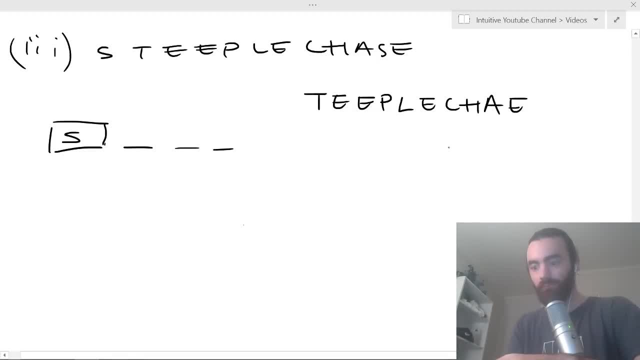 into account. so taking away the e's and just thinking about the final letters that we have, tpl, ch a. so let's take the case where we've got zero e's- right, so we've got zero e's. well then, there's from this, from the remaining letters we've got. 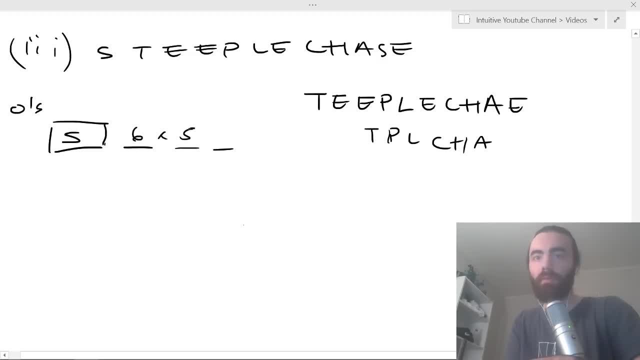 one, two, three, four, five, six. so there's six different ways times and then five different ways times in four different ways. and remember, if we let's say tpl, we calculate tpl, i mean pick tpl. well, this is the same as lpt, which is the same as you know. it's the same thing. 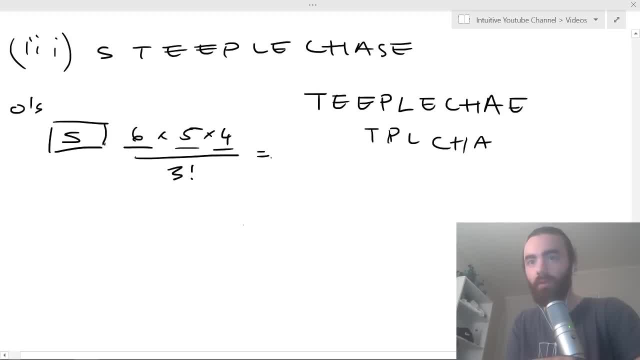 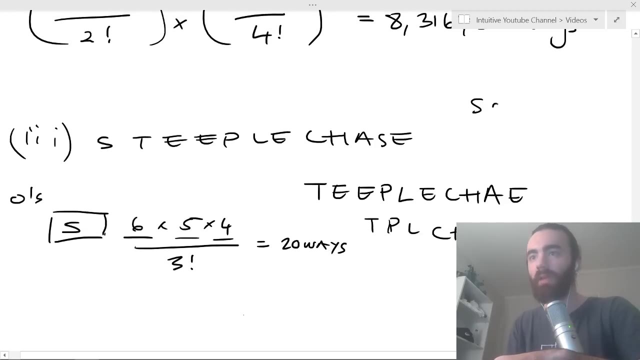 so then we have to divide by three factorial. that equals. so for zero ease, there's no ease pick. and then six times five times four divided by three factorial. so there's 20 ways to do that and i hope it makes sense that why i'm taking out the ease, because look if i pick s e. 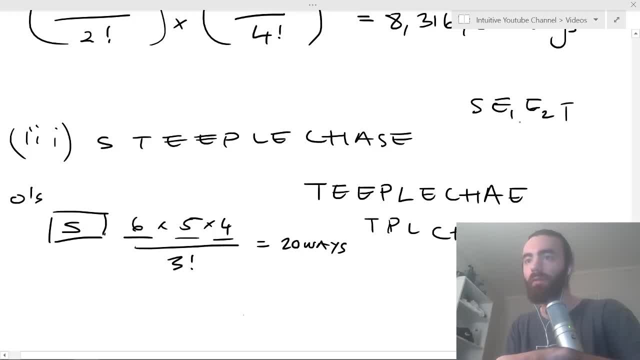 one e, two, t, like. that's the same we we're counting. if we were to do it like i said before, like with a ten thousand, oh well, then we're also counting three, two, we're also counting four, two, like if these ease will be one, six, obviously, there's one, eight, and then three, two, two will be the second eight. 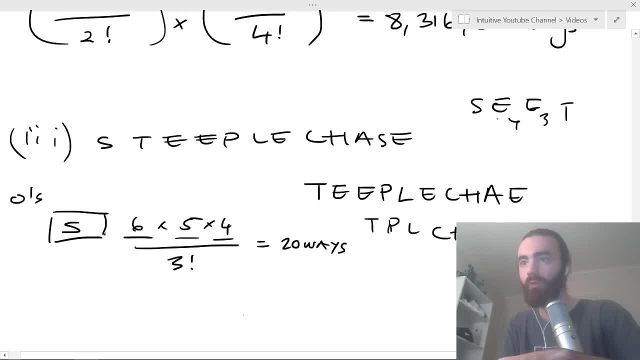 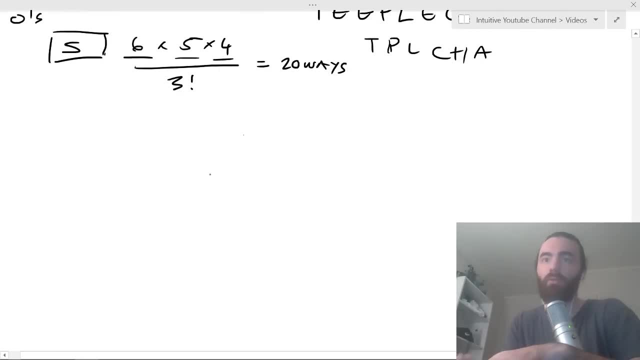 two's. that's just the same thing. we're just using fifths, that сок in sort in the middle we're taking. e's are different for three. we can't. we're over counting by all these different e's. they're all the same selection. so we're over counting by a hell of a lot. so we need to be careful and be. 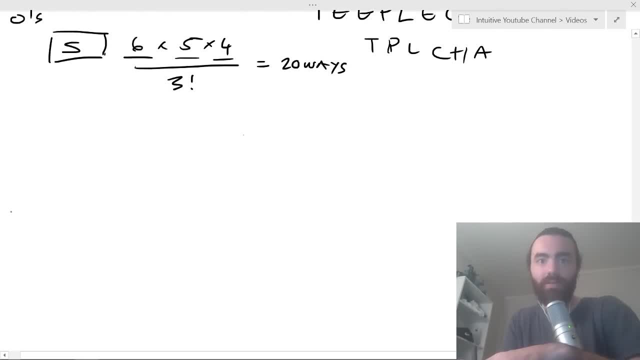 more specific and focus on each case, each case. so let's say, if we pick one e here, remember we've got this fix s and then we've got these three slots, but then we've picked one e. there's only one way to do that. right, there's one e we're just picking. we're saying this is the case where there 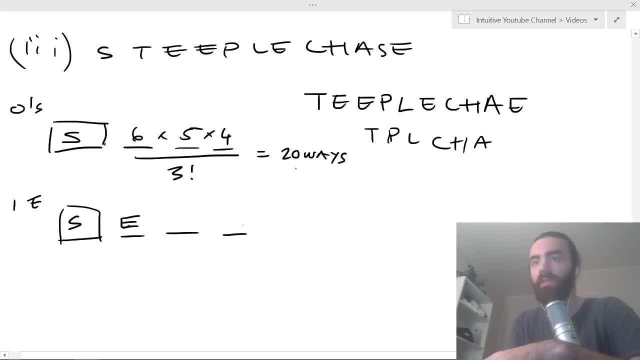 is an s and there is an e, and now we have two slots and we have six different ways to pick these letters. so six times five, divided by two, factorial, which is 30. divided by two, which is 15- all right for that scenario- and then two, two. how many ways can we do it when we select two e's? 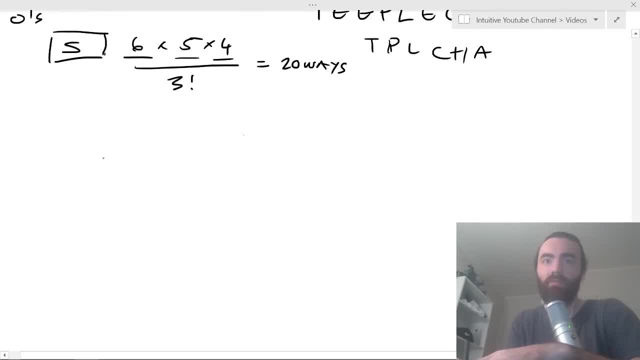 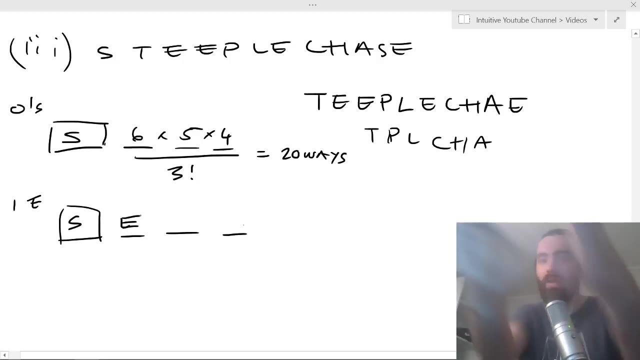 a hell of a lot. so we need to be careful and be more specific and focus on each case, each case. so let's say, if we pick one e here, remember we've got this fix s and then we've got these three slots, but then we've picked one e. there's only one way to do that. right, there's one e we're just picking. 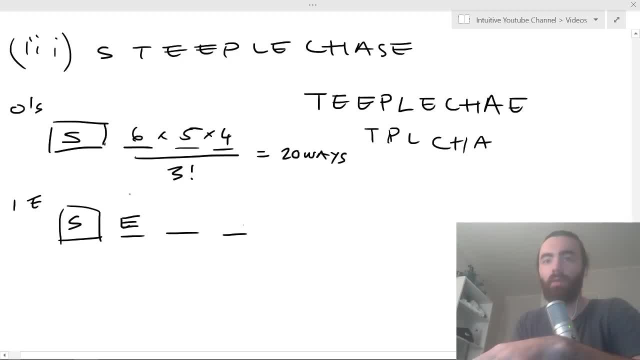 we're saying this is the case where there isn't and there isn't e, and now we have two slots and we have six different ways to pick these letters. so six times five divided by two, factorial, which is 30, divided by two, which is 15.. 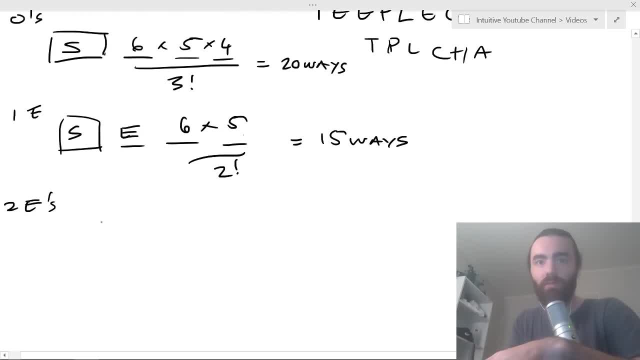 all right for that scenario. and then two, two. how many ways can we do it? when we select two e's, that's e, e, and then we have a final slot. well, there's six letters and one slot, so there's just six different ways to do that. but also, you've got to remember this last one. well, if we select 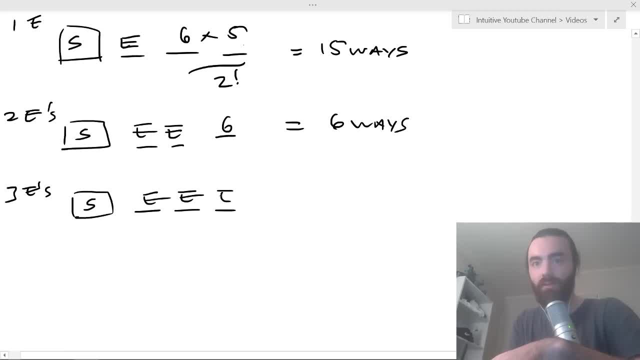 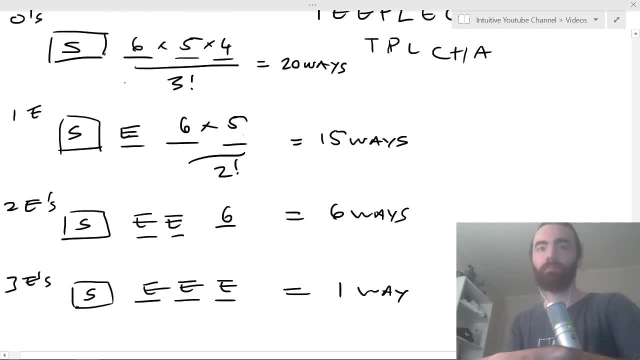 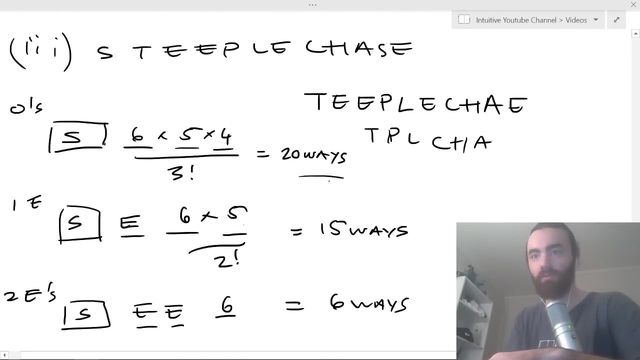 3e, two, three. how many ways is there to do that? one way, there's only one way to do that, right and now. so for each of these cases, we now add them up right. so we say: well, for the zero ease there's. how many ways can we um different selections of these uh letters can we make? the zero ease is 20. 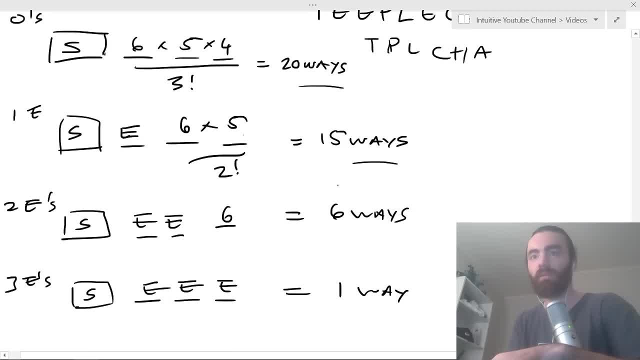 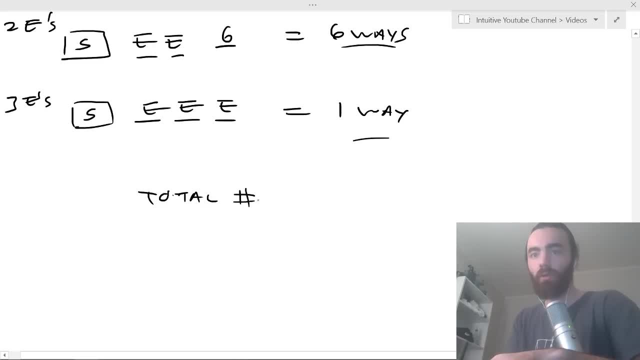 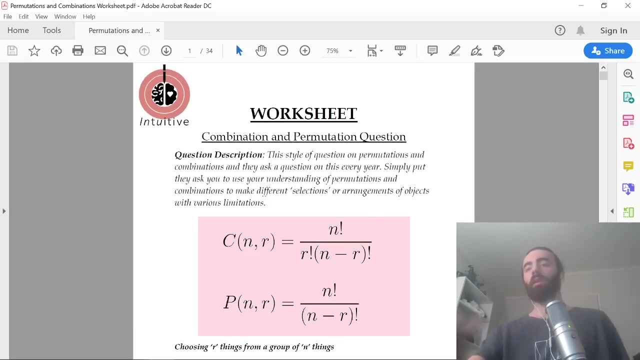 plus the number of selections we can make for one e, which is 15, so it's 35, 41, 42. so the total, so total number of ways, is equal to 42 ways. okay, that's the answer and that's it. so. yeah, so you got the worksheet, like i was saying before, go through these questions, get. 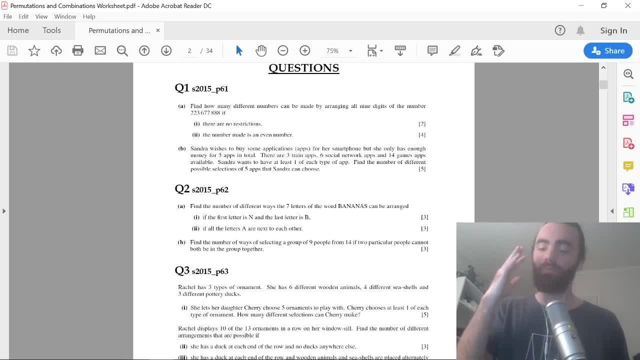 a feel for them and your brain will start to recognize the patterns. and don't don't yourself, you know. if you don't understand how to do it, then look at the answer and try and understand the answer. and try at understand the answer, try and understand how the hell do they get there. and if you don't, you can. 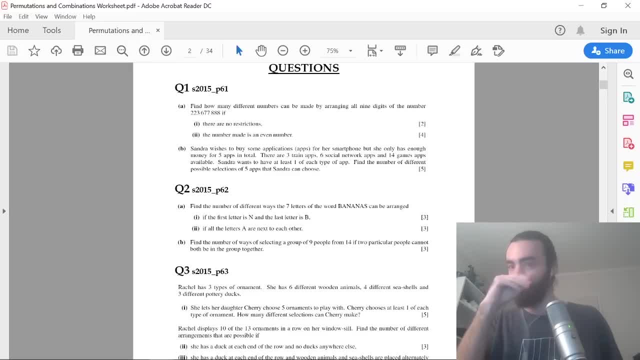 come here and ask in the comments and I'll. I'll answer and other people will answer and just help each other. get good at this question together. you know, two brains are better than one man, and yeah, that's pretty much it. there's nothing. this is the end of the series and I'm done with. 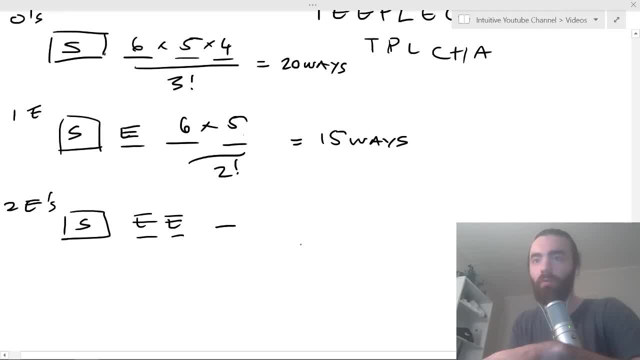 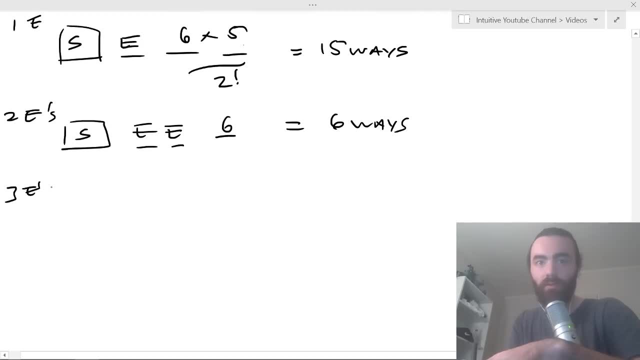 that's e, e, and then we have a final slot. well, there's six letters and one slot. so there's six different ways to do that. but also you've got to remember this last one: well, if we we've got select three e's, two, three, how many ways is there to do that? one way, there's only one way to do that. 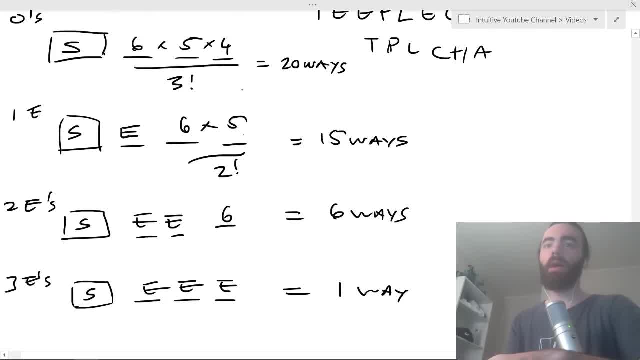 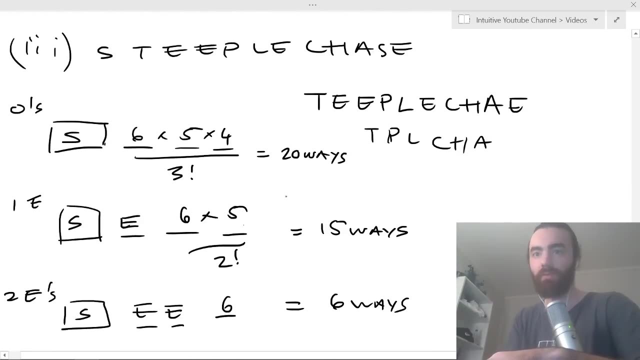 right and now. so for each of these cases we now add them up right. so we say: well, for the zero e's there's: how many ways can we um different selections of these uh letters can we make? the zero e's is 20 plus the number of selections we can make for one e, which is 15, so it's 35. 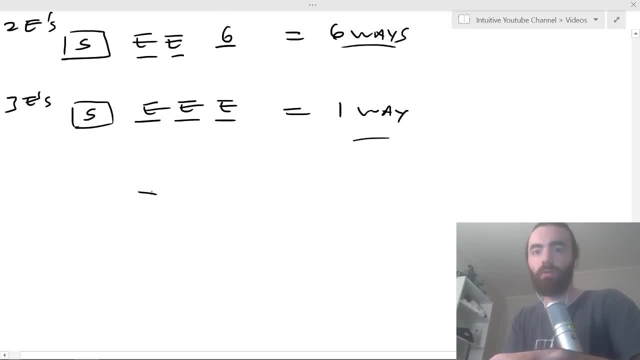 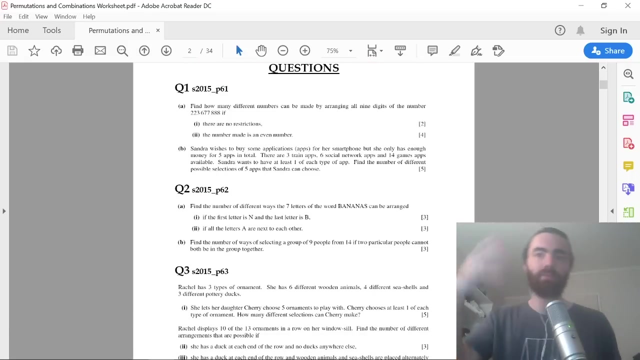 41, 42. so the total. so total number of ways is equal to 42 ways. okay, that's the answer and that's it so yeah, so you got the worksheet. like i was saying before, go through these questions, get a feel for them and your brain will start to recognize the patterns. and don't, don't, bullshit. 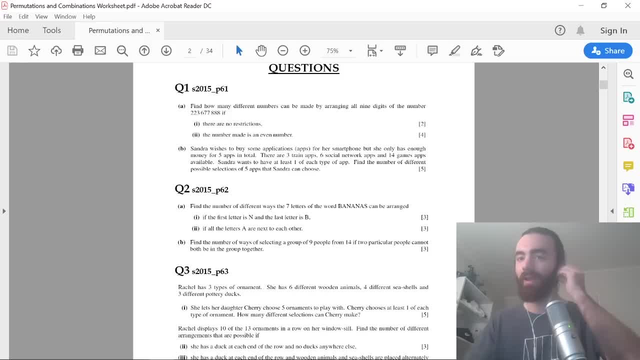 yourself. you know, if you don't understand how to do it, then look at the answer and try and understand the answer. try and understand how the hell do they get there. and if you don't, you can come here and ask in the comments and i'll i'll answer and other people. 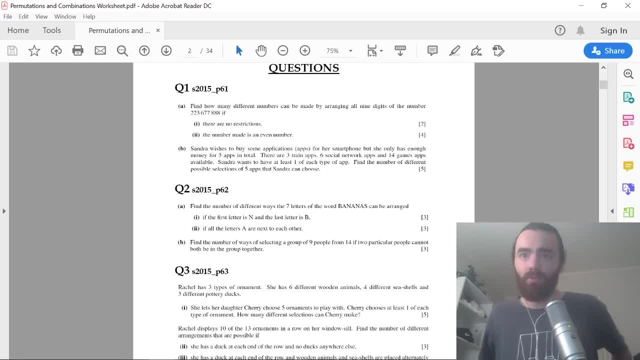 answer and just help each other. uh, get good at this question together. you know, two brains a bit in the one man, and yeah, that's pretty much it. there's nothing. this is the end of the series and i'm done with statistics, thank god. and um, yeah, like, what else do i want to say? like 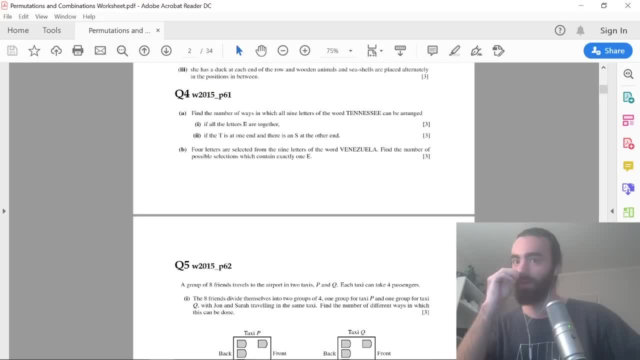 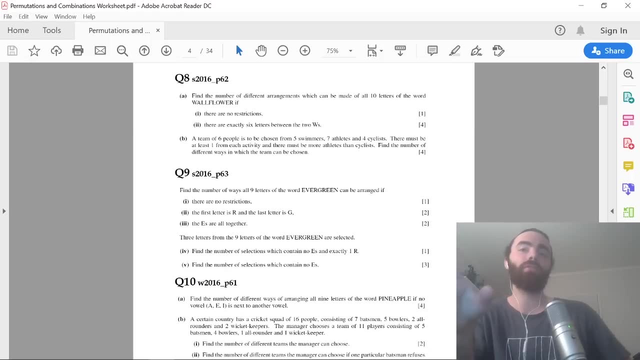 honestly, these videos, if i'm being honest, are getting repetitive for me and stuff like that, but my really my reward here is this: this really does work and for for use for you, of the those of you who actually take this seriously and do this approach, where we, you know, we group similar questions together and then you go through. 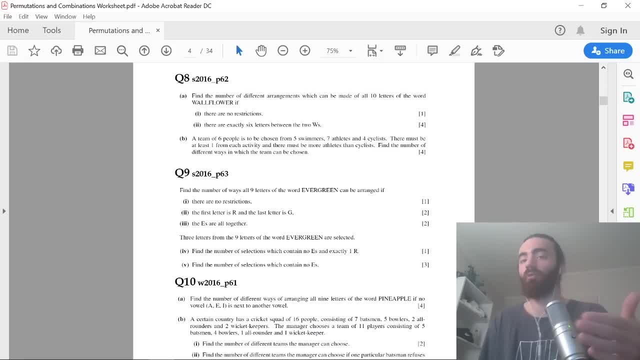 and then, when you sit in your exam, you do get an incredible grade. that's my reward for doing this, even though it can be a bit boring for me and a bit repetitive. my reward is: look, when you do get a grade, that makes me happy because this, this really does work. i'm telling you it's going to work. 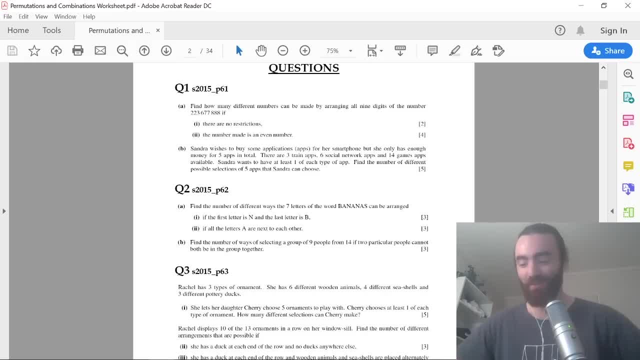 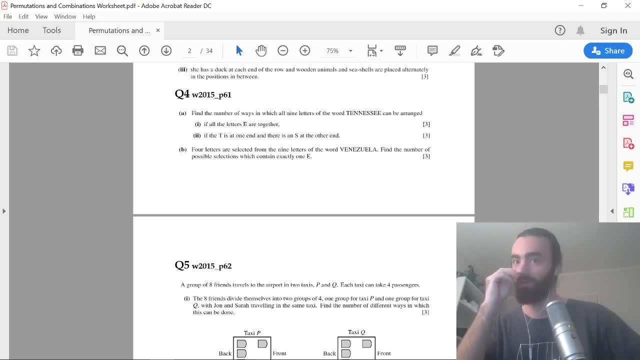 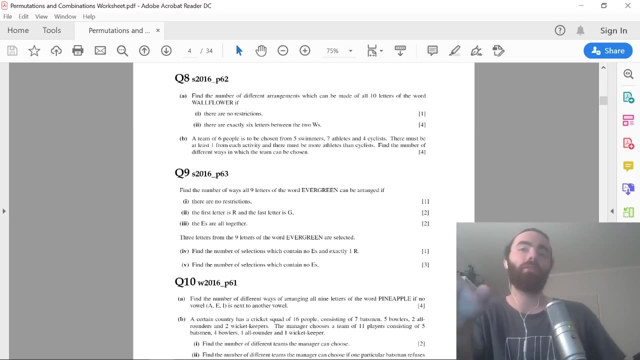 statistics, thank god, and yeah, like, what else do I want to say? like, honestly, these videos, I'm being honest, are getting a bit repetitive for me and stuff like that. but my, really my reward here is this: this really does work and for you, for you- of the those of you who actually 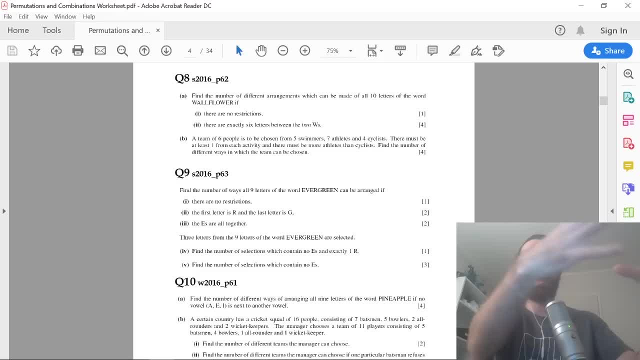 take this seriously and do this approach where we, you know we group similar questions together and then you go through it and then, when you sit in your exam and you do get an incredible grade, that's my reward for doing this, even though it can be a bit boring for me and a bit repetitive. 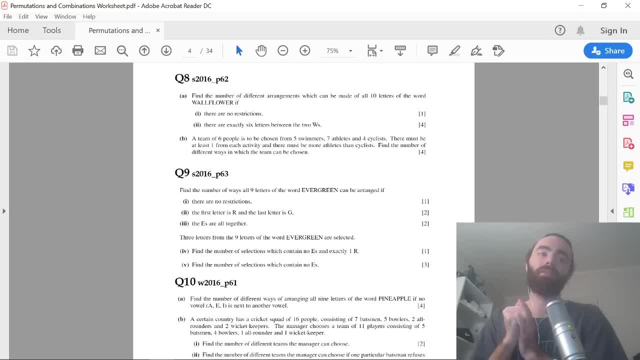 my reward is: look when you do get a good grade. that makes me happy because this, this really does work. I'm telling you it's going to work. you're going to feel like you're in the. you're in the matrix. 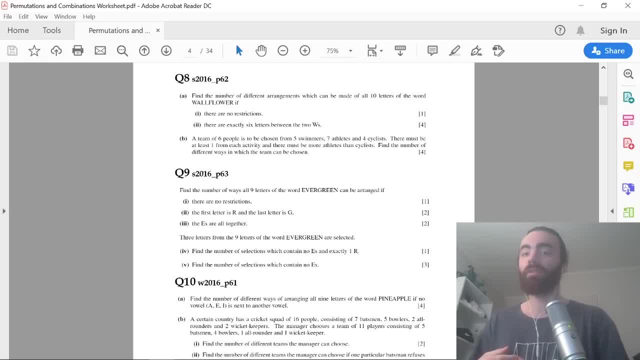 if you take this seriously and you put energy into this way of approaching exams, when you get into your exams you're going to. you're going to. honestly, if you've gone 100 on this, you're going to think you're in the matrix. you're going to be looking at your exam like I know exactly what to. 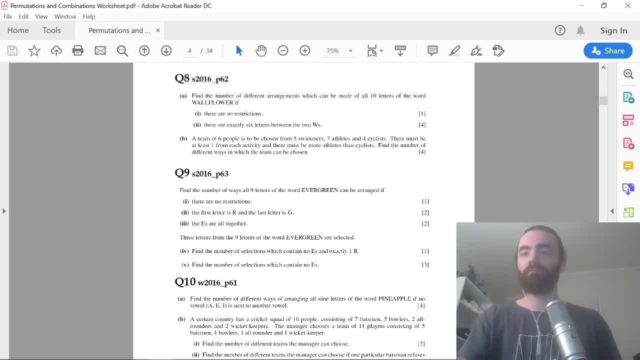 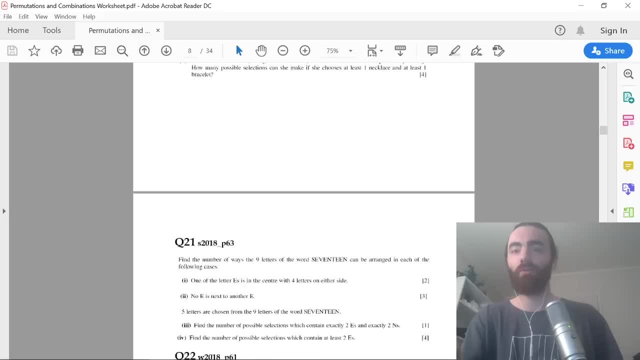 do everywhere. your brain is just going to be like boom. so yeah, anyway, that's it. download that, start going through it and, yeah, I'll see you. I don't know what paper I'm going to do next, but 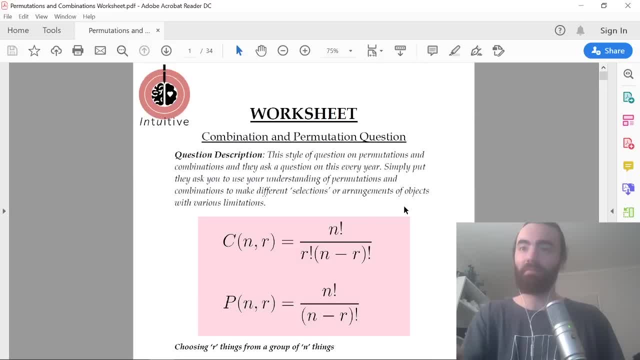 yeah, I'll see you when I see you in whatever video I'm making peace out.